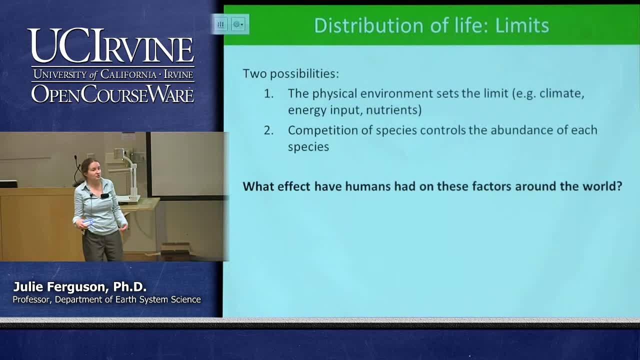 And we talked about what might limit the population of humans on Earth, what might set our carrying capacity for humans on Earth. And then we also talked about the second thing, the competition of species. So if two species have to coexist in the same area and they have the same requirements, 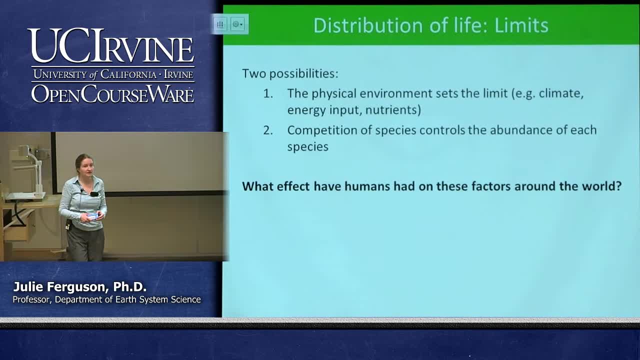 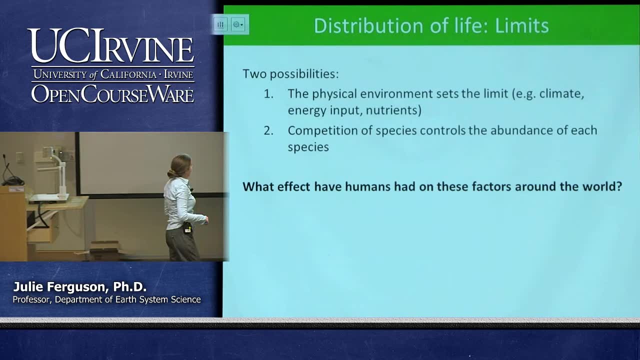 one of them is always going to be out-competed, One of them is always going to do better and push out the other, And so I didn't have a chance to ask this question at the end. But what effects have humans had on both of these? So what effect have we had on the second? 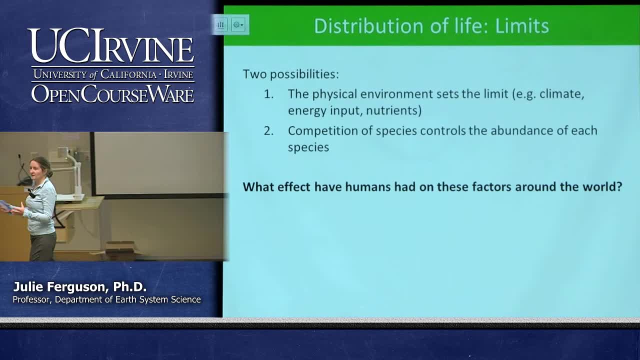 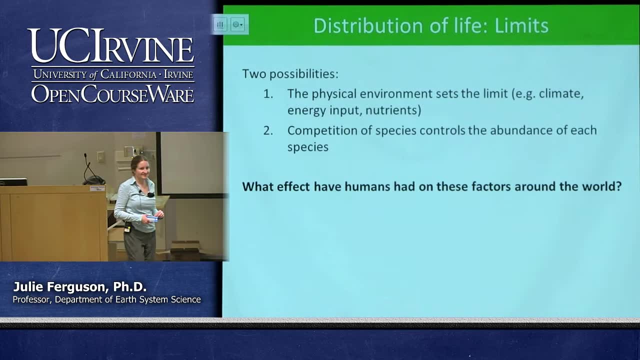 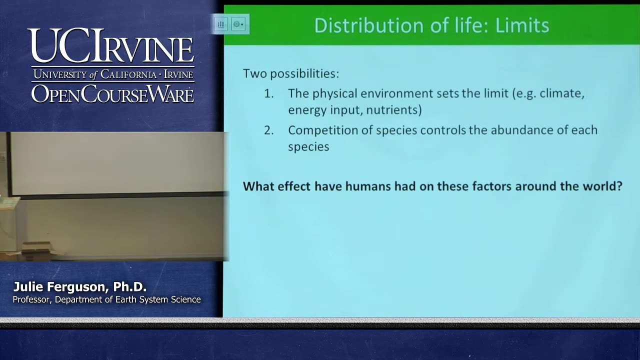 of those. Can you imagine what effect that human populations have had on the competition of species? What have we done? Yeah, Interesting, Absolutely. We've massively changed. So, for example, in Australia we introduced cane toads, And cane toads have taken over and there's no real natural predators there. 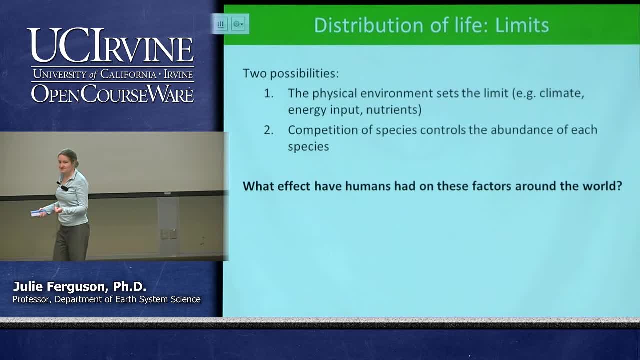 And they're pushing out other species. The big one, of course, is rats. Rats were introduced whenever ships landed on different islands, And rats have done enormous damage to previously isolated populations with their own species. Not only that, but plants, So around here. 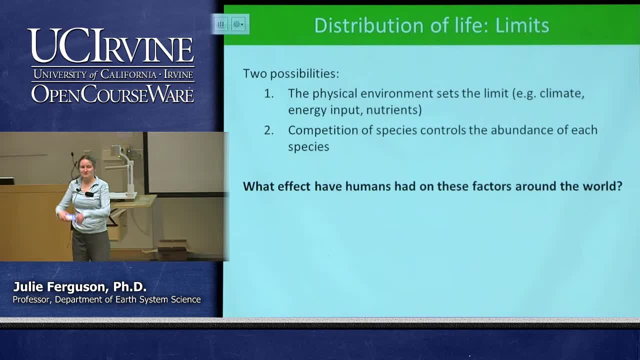 Very few of the plants you see out there are actually native species. Those beautiful eucalyptus trees don't really belong here. We planted them here And so we've seen very, very different switches And there's a big push now to try and remove a lot of that non-native vegetation. 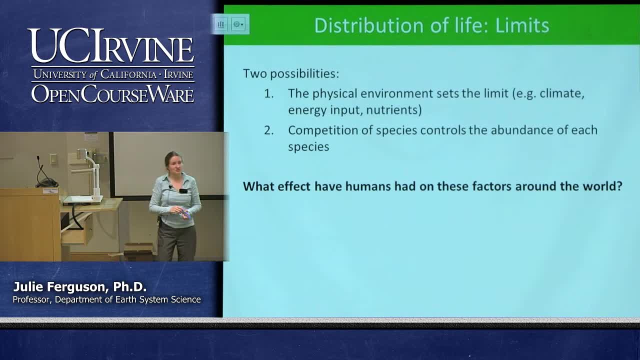 especially if you ever go out to the Channel Islands National Park just offshore here, Then they've put a lot of effort into trying to get significant proportions of that national park back towards its natural vegetation And you can volunteer in the summer, You can go out and they'll set you to sort of removing some of this invasive vegetation. 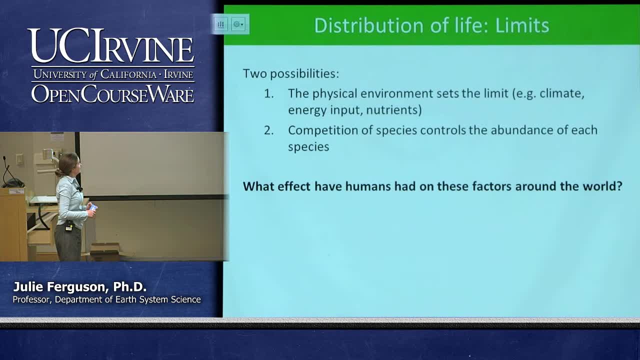 because it's a long process, It's not an overnight thing. So we've definitely affected the species diversity around the world just by introducing competitors, reintroducing animals where they shouldn't be. And the more obvious one is: what have we done to things like the nutrients or the energy inputs for ecosystems? 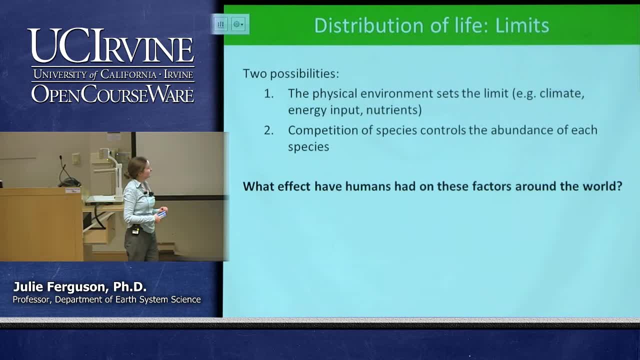 Do you think as many animals can exist now on Earth, now that there's sort of 7 billion of us? No, Because, remember, we are actually sort of taking up sort of over 20% of the net primary productivity of the world, And so that energy comes to us. 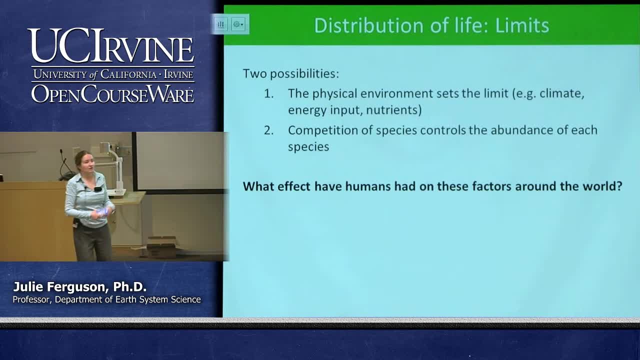 It's less available for other organisms to use. And not only that, but we're doing things like we're changing the composition of the atmosphere, which changes Our climate, which shifts around rainfall patterns and temperatures. We're also doing funny things to nutrient variability in different areas. 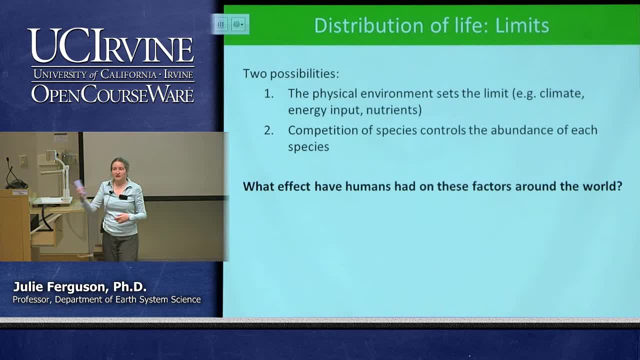 For example, where we're farming, we might be adding more nutrients, In others we might be seeing less. So we've done an awful lot to change these patterns around the world, And so of course, we're seeing changes in the biosphere. 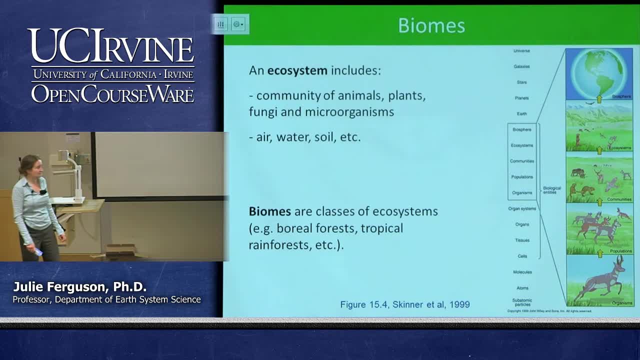 So I'm going to talk briefly about biomes at the beginning today, And this is just a reminder that when I talk about ecosystems, I'm not just talking about the different organisms there. I'm also talking about the non-living components, So things like the atmosphere, the water or the soil. 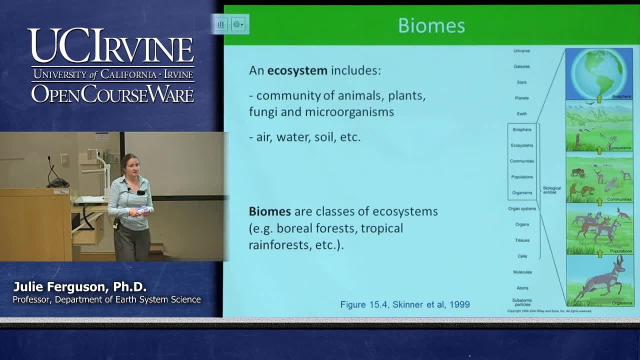 And biomes are just sort of we lump together different ecosystems. So if we have different, subtly different types of sort of tropical forests, we might lump them together and call them tropical rainforest. It's sort of a way of simplifying our biomes. 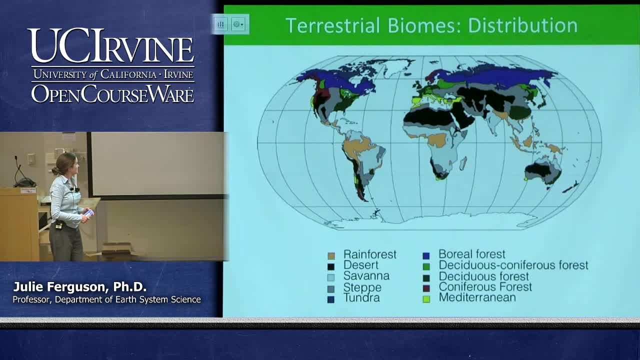 And I wanted to show you a little map of where our biomes are. So here are some. These are some of the big ones, So have a look. Which biome are we Find Irvine on the map. What biome are we Mediterranean? 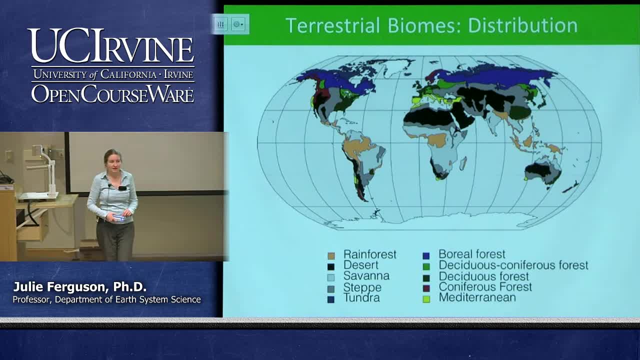 Yeah, And we're pretty rare. If you look, there's not a lot of Mediterranean climate around the world. The only other place really is the Mediterranean And little bits perhaps along the southern tips of our southern hemisphere continents. But you can see that we have enormous amounts of boreal forest. 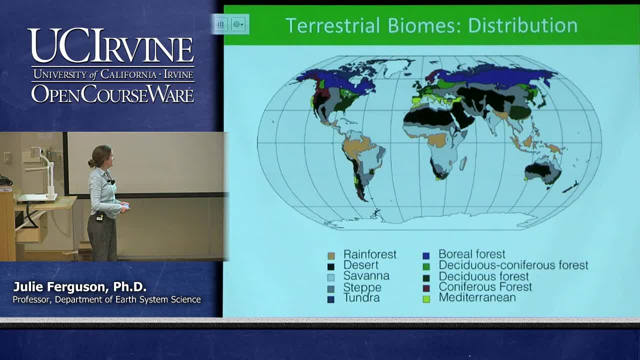 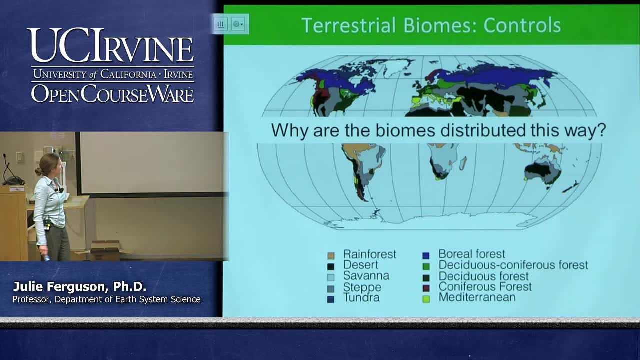 We have sort of large amounts of other sort of different types of forest- coniferous, deciduous- And then sort of, as we get towards the pole, we get things like tundra. So my question for you, which sort of basically, is what we did on Friday? 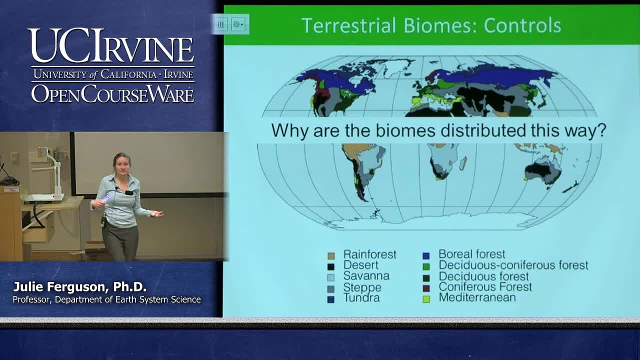 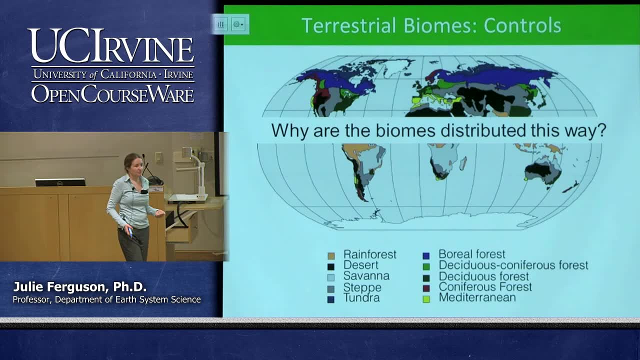 is: how do we? what really controls these different types of biomes? So what were some of our controlling factors on our biomes? Why do we not have tropical rainforests on Greenland? It's not a complicated question, I promise Yeah. 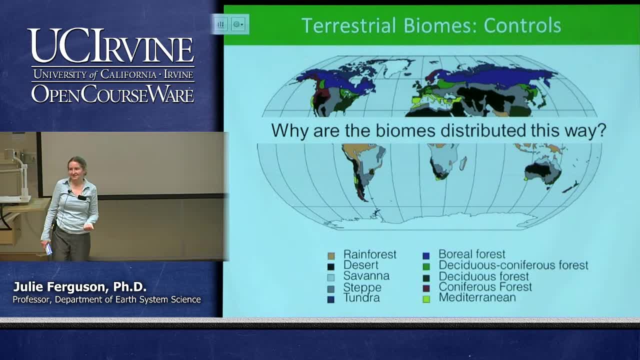 Temperature, Yeah, Temperature Okay. So temperature affects our sort of distribution of our biomes. What else might affect? Why do we not get tropical rainforests in the Sahara? Sunlight, Some sunlight, definitely- So closer to the poles, when it's dark for a lot of the year, the plants have to be more adapted. 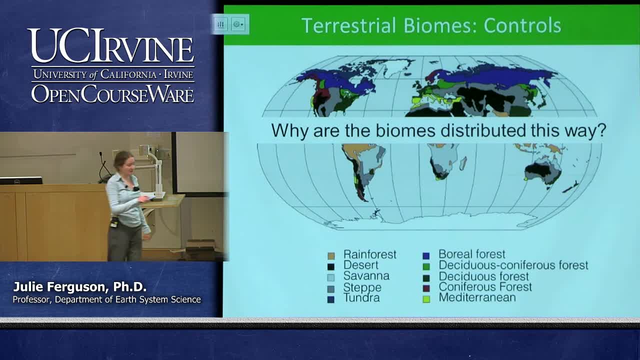 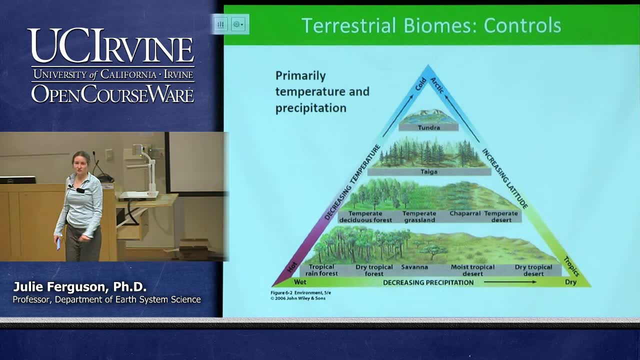 But about rainfall, the other one, that's sort of the big one. So our biomes are really distributed this way Because of Precipitation and temperature, So we can draw ourselves a little nice triangular diagram. We're sort of wet in this left-hand corner and dry in that. 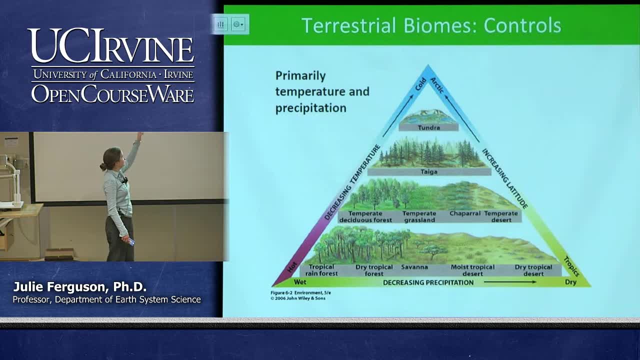 And then we sort of move towards the pole or we decrease our temperature towards the top And we can sort of lay out these different types of biome on that map, really, And these are our major ones, And when we have different biomes like this: 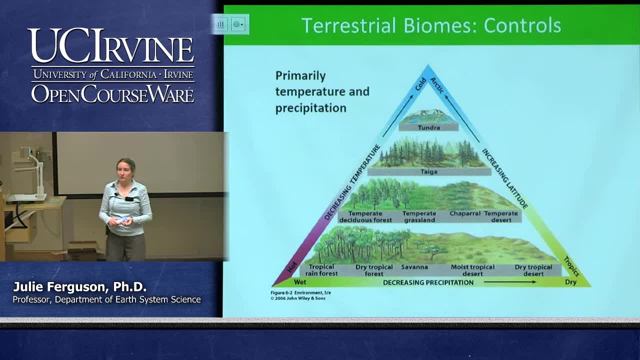 you can imagine that each of these areas has very different net primary productivity. It was one of the questions I think. I asked Sort of how much biomass really is there in a system? How rapid do you think growth will be? So where do you think? 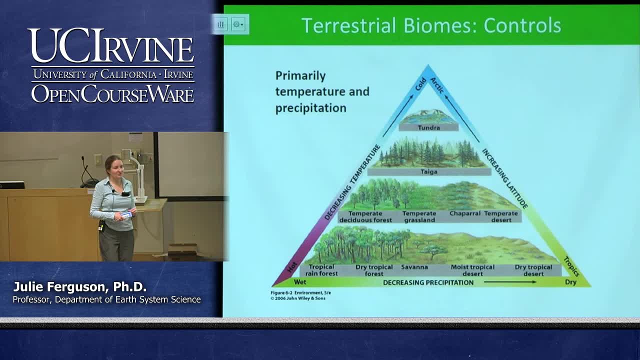 Which corner do you think there will be most net primary productivity? You can point if you like. Oh, my goodness, Come on. I know it's Monday, but This one tropical rainforest, This is probably more where there's going to be a higher net primary productivity. 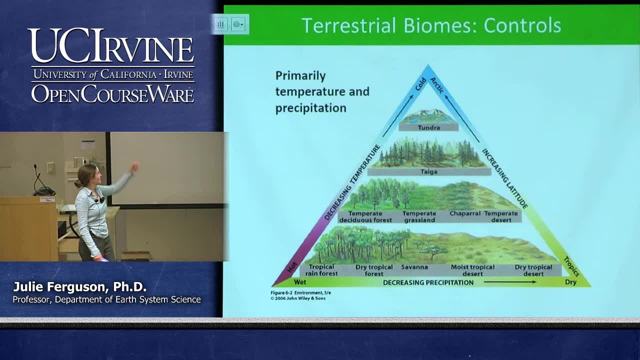 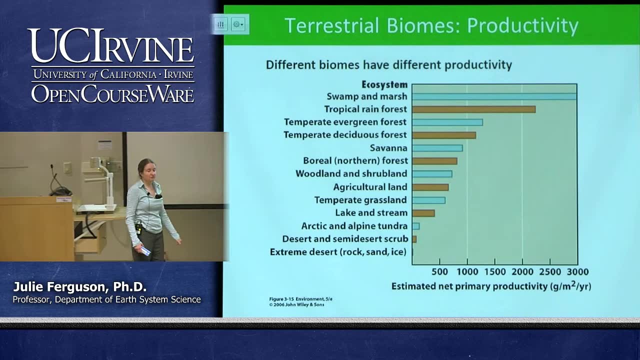 And as we get Drier, our rainfall is restricting that. As we get colder, our temperature might be restricting that. And so here's a little graph showing you the different productivity of these different types of biome. And so marshland isn't necessarily on the previous diagram. 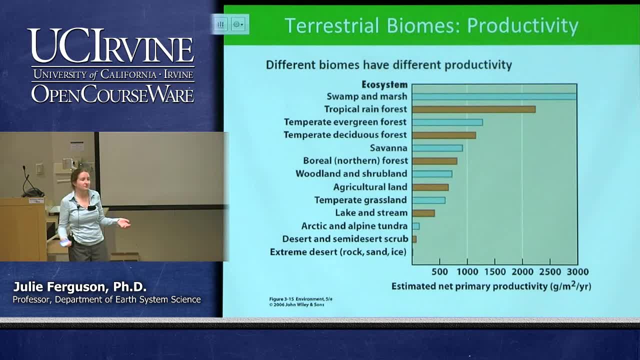 but I included it here because it's actually one of the most productive types of biome on an ecosystem on the Earth. And then you can see, as we get into sort of extreme desert, into tundra, we see that we have a lot less primary productivity. 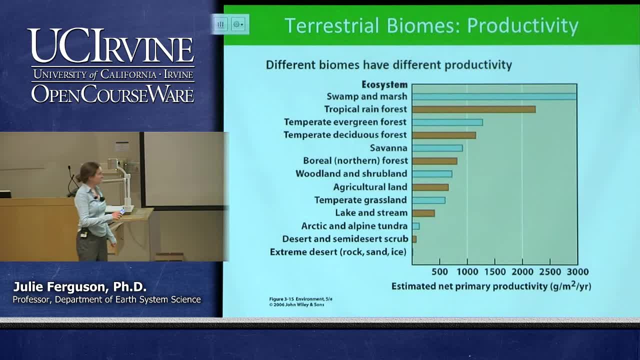 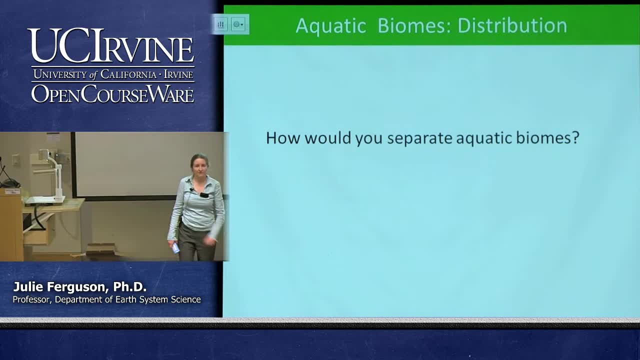 which makes sense because we're limiting ourselves. Okay, So I talked about these terrestrial biomes and how we separated them out. We have rainforest, we have tundra and we have these different limiting factors. So aquatic biomes, things that live in water, 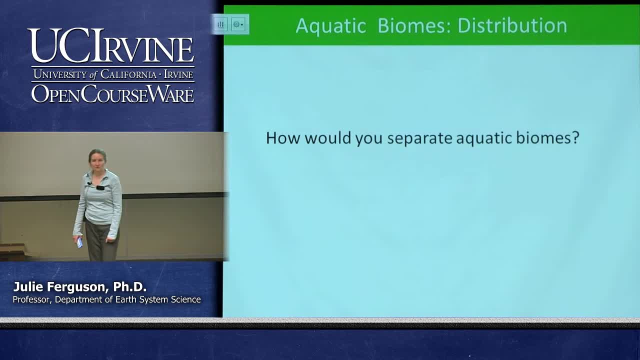 How would you go about separating out? So, with rainforest, we had big giant trees and we had lots of rainforest, We had rainfall and precipitation, But what about aquatic biomes? What's the first thing that you would do to separate out? 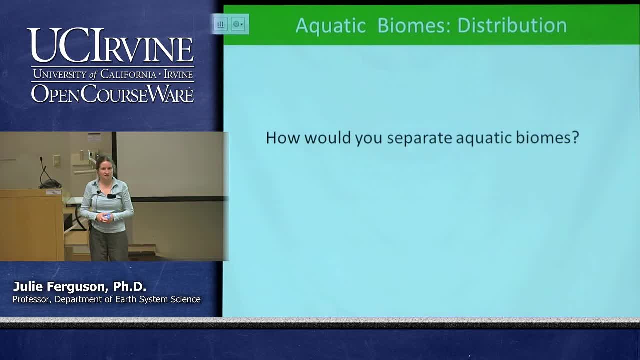 and talk about different biomes in the aquatic world. Pressure- Sorry, Different pressures, Quite possibly. So absolutely. And where do we get different pressures? mainly Since you go down, you get more pressure. Yeah, So different pressures. So some of the organisms that live really deep down in the ocean are very adapted to that. 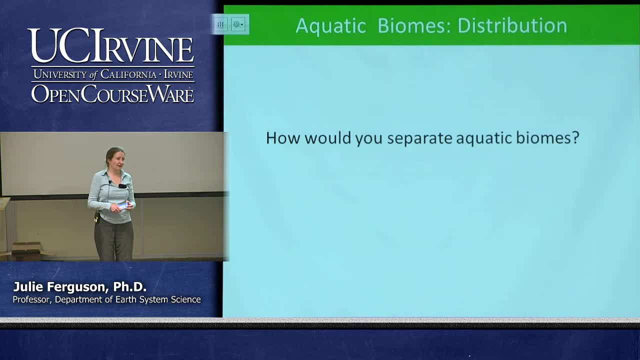 And when the poor things are caught and brought up to the surface, they don't do well, They're sort of bleh And so definitely pressure is one of them. What's the big two? You can separate it into well Precious. 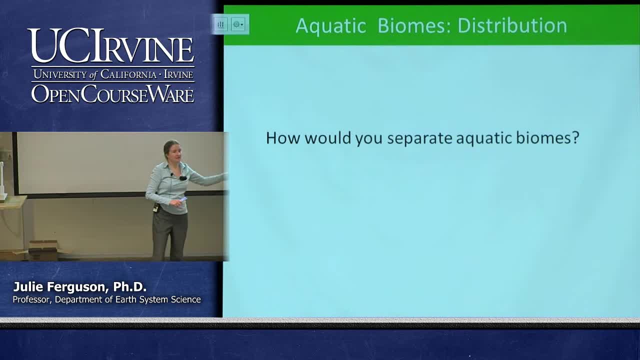 Absolutely So. salinity. So freshwater aquatic biomes are very different from sort of the ocean aquatic biomes. So salinity is a big one And we actually separate that into three. We have sort of salty ocean, We have freshwater, We have that transitional in the middle. 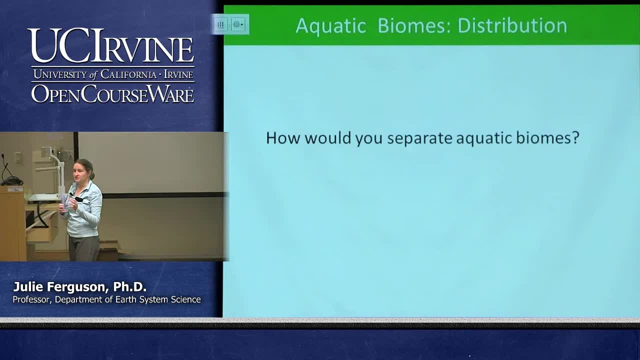 So things like estuaries. So things like estuaries or sort of swamps or marshes or mangroves at the edges where that freshwater is meeting our salinity, And then we definitely had pressure. What else might affect the distribution of life in the oceans? 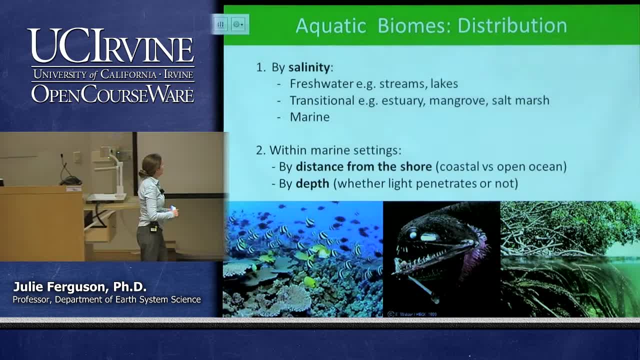 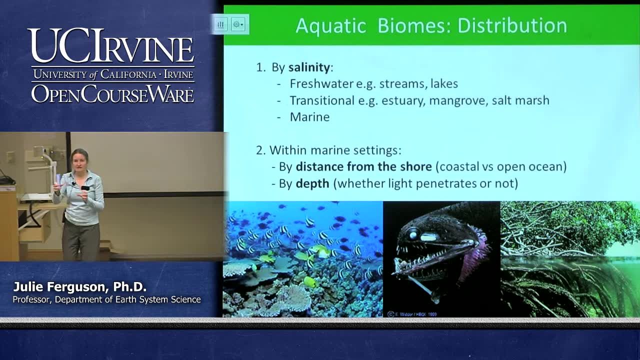 Energy from sunlight- Sunlight, Absolutely Okay. So by salinity is our first way that we would separate out our aquatic biomes and create little distinct groups. But also within marine settings we have things like pressure and sunlight, So creating differences in the aquatic biomes with depth. 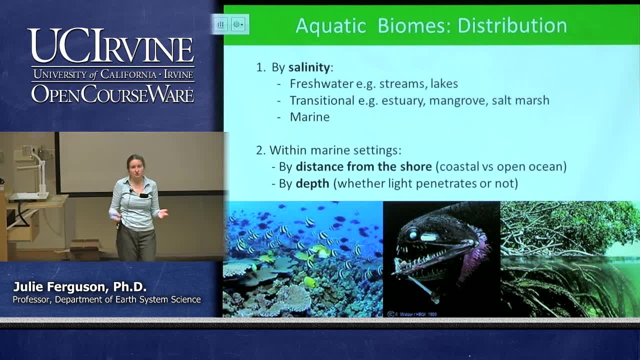 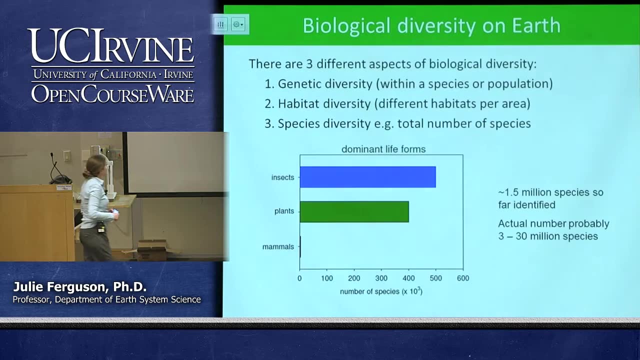 But also things like distance from the shore- Are things coastal or are they more open water environments, And we get different types of organisms in that way as well. So we can keep on subdividing as much as we like, But these are really the main ways we go about doing that. 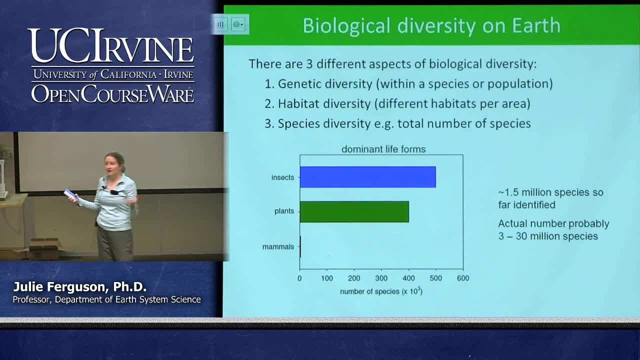 So now I wanted to talk about biological diversity, because the idea behind all of these different biomes is that they're differences. We have diversity. We have diversity in terms of even genetic diversity within a species. We have habitat diversity. We have different environments on Earth where organisms can live. 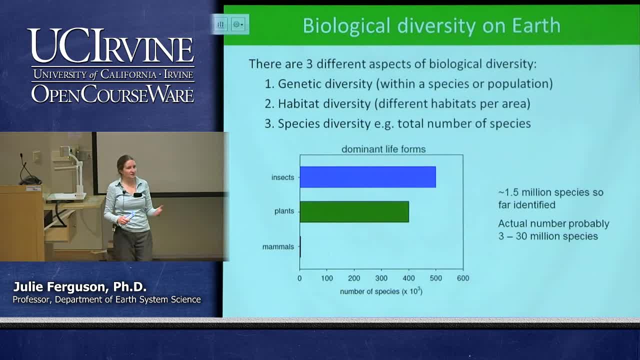 And we also have species diversity, which is more what we think of. when I talk about diversity, You think of just the total number of different species that we see on Earth, But often these are tied in together, And if we look at what's alive on Earth so far- or today rather, 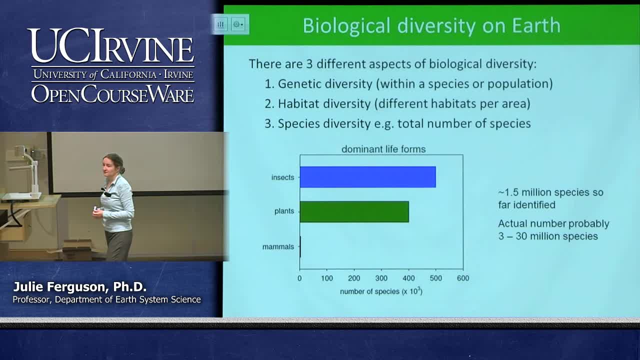 we have maybe 1.5 million species that we've identified And that's a lot, But we haven't even come close to probably describing the diversity that exists today. Somewhere between 3 and 30 million species actually probably exist on Earth today. 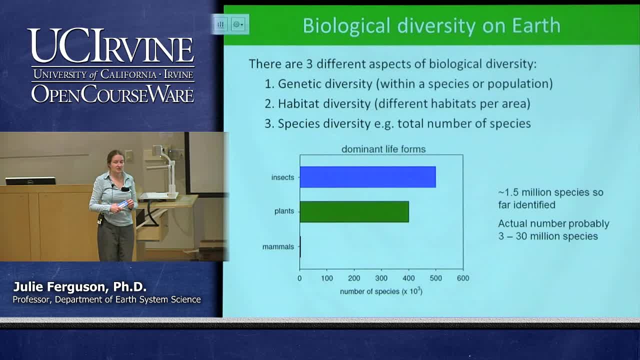 And we just haven't described them yet, And we're still discovering new species today, And not just of mammals. okay, Because I wanted to show you. This is the number of species that exist for mammals, and then for plants, and then insects. 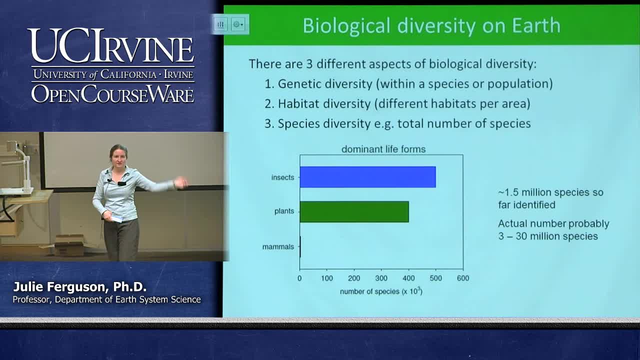 A lot of our diversity isn't in the giraffes versus the elephants, versus gorillas versus mice. It's actually in the insect populations and in the plant populations. So the diversity that we tend to see is just a fraction of what's out there. 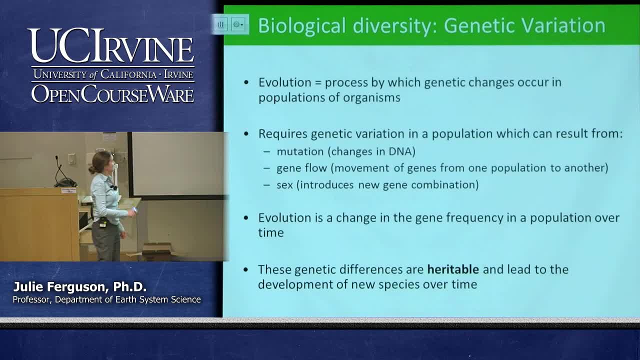 So what I wanted to talk about now is really how we get that diversity, And so we're coming on to evolution. So for evolution to work, evolution is really this idea that we see genetic changes through time in organisms. okay, And in order to get genetic variation, we need to have genetic variation to begin with. 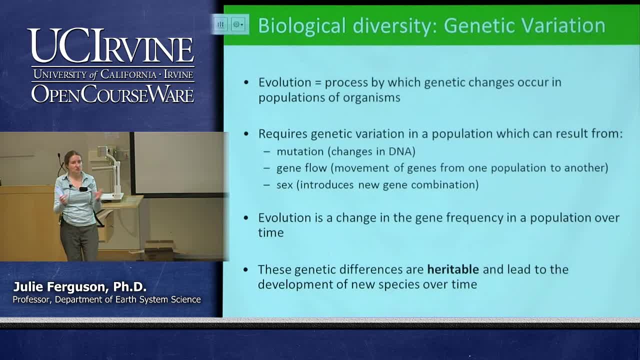 If we're going to shift the proportions of genes, we need to make sure that we have genetic variation to begin with, And so some of the ways that we can create genetic variation is by mutation, So just changes in our DNA, And we'll talk more about that. 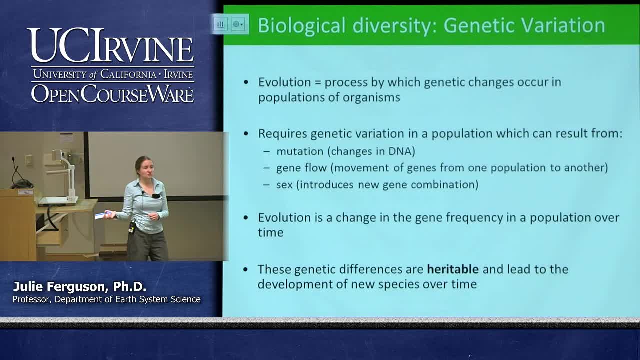 We'll talk about that in a second Gene flow. So if you introduce sort of an organism from one population to another population, they would introduce new genes into that new population. And also by sex you introduce different gene combinations together And so you're creating genetic diversity. 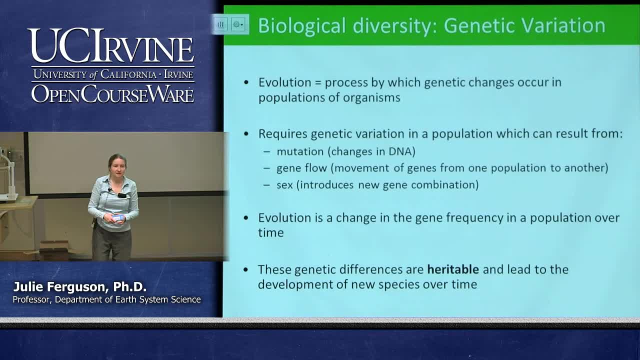 And so what we talk about when we talk about evolution isn't just that we're not creating better species. That's not how evolution works. What we're saying is that, one way or another, we shift the proportion of genetic material in our species. 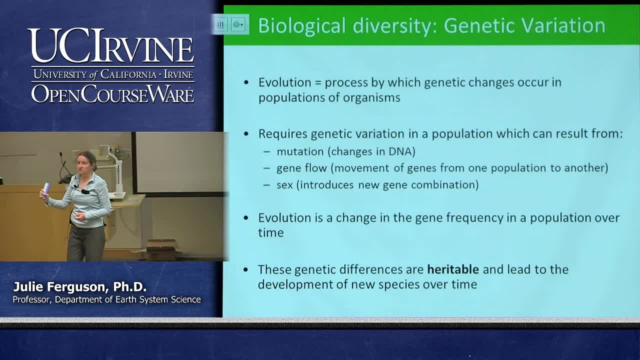 And the idea behind this is that that genetic material is heritable. So if you see genetic variation in the parents, then that will be inherited by their offspring And so through time we get successive changes to our genetic code And that over time when that's sort of large enough. 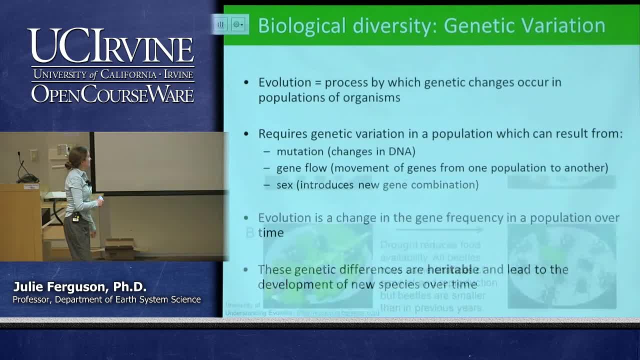 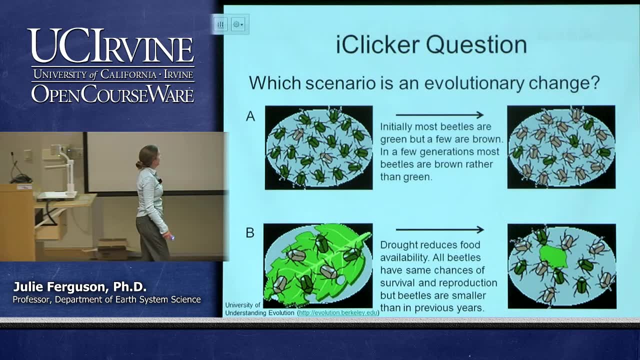 we can end up with new species at the end. So let's have a look at my first question of the day. So I have two different scenarios here. Scenario A is that initially most beetles are green but a few are brown, And in a few generations most beetles are brown rather than green. 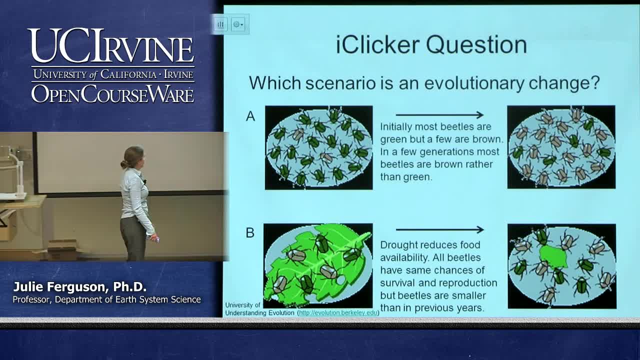 In my second scenario, drought reduces the food availability. All of these beetles on the left have the same chances of survival and reproduction, But the beetles in the north have the same chances of survival and reproduction And the beetles in the north in the next few years are smaller than in the previous years. 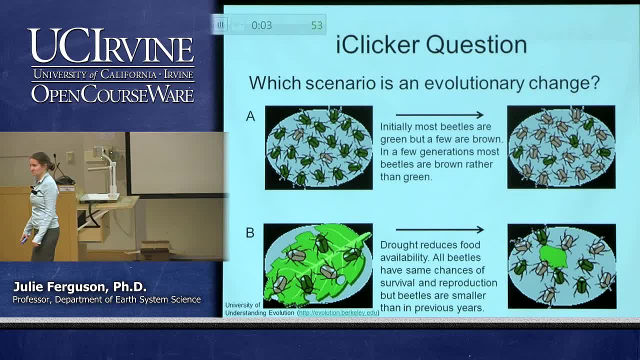 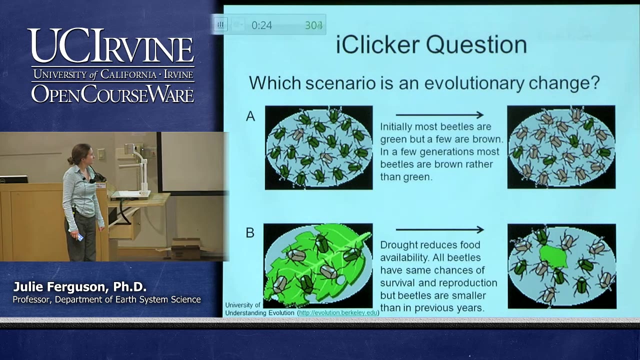 So which of these is an evolutionary change? You can ask your neighbour or debate it if you would like. Scenario B is that most beetles are green, but a few generations of beetles are brown. A couple more seconds. Scenario C is that most beetles are green, but a few generations of beetles are brown. 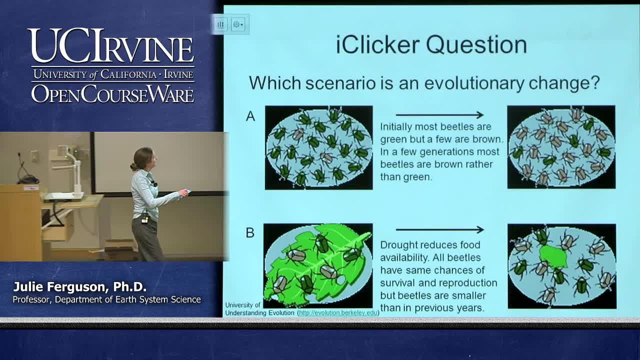 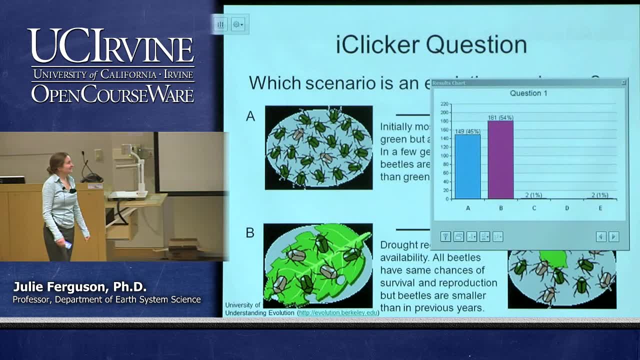 Right, so let's take a look and see how we're doing on evolution. Scenario D is that most beetles are green, but a few generations of beetles are brown. OK, so we have more or less a 50-50 split. 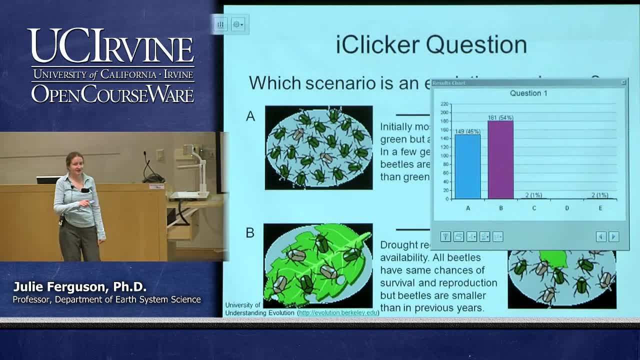 So there wasn't very much talking in the room And I want you to turn to the people behind you or to the side of you or in front of you and convince them why you're right. OK, explain to them. So remember, an evolutionary change is a genetic change in the population. 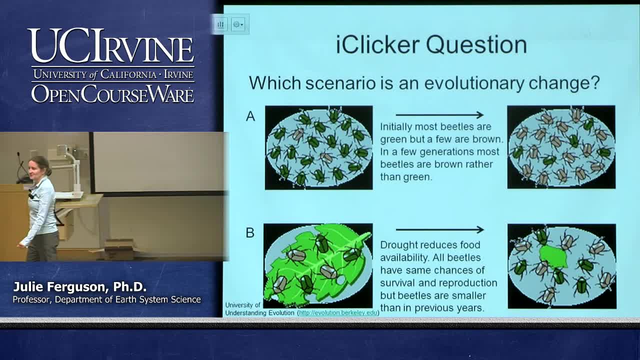 So turn to them. I'm going to give you one minute to convince your neighbours why you're right, and we'll see if we get another shift. SCARLET CHILDREN- CHIRP. SCARLET CHILDREN- CHIRP. SCARLET CHILDREN- CHIRP. 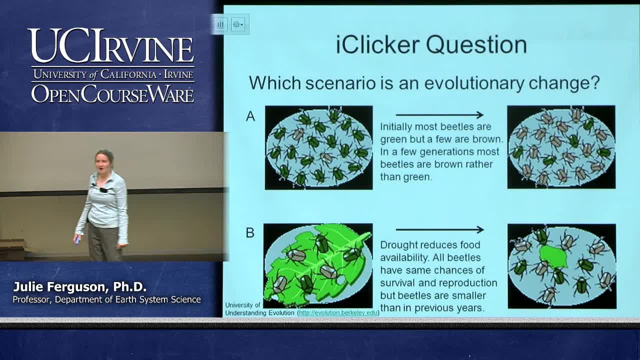 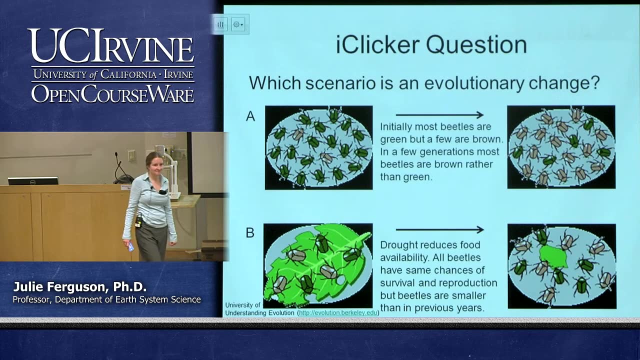 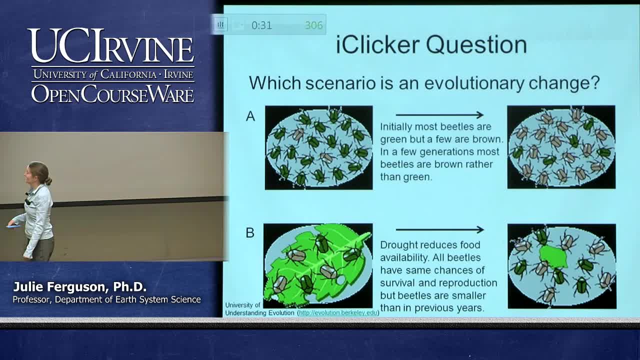 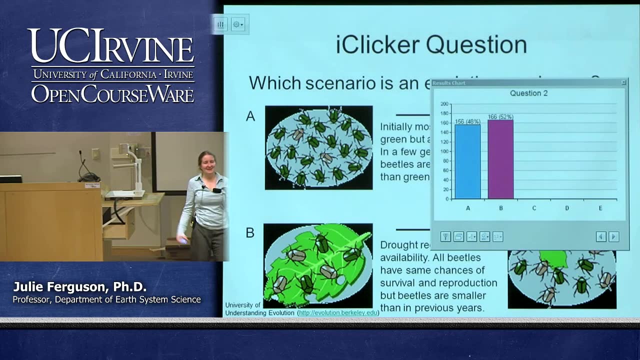 We're missing quite a few votes. I'll give you a couple more seconds. Let's take a look and see how persuasive you guys are. So either everyone switched or no one switched- Okay, you're stubborn. So, in fact, the majority in this case are not correct. 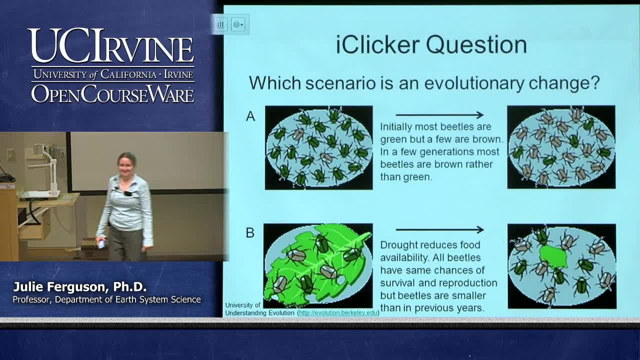 I know So it is A, So let's have a think. Let's have a think about this, given that there is such a change. So, with B, remember that all my beetles have the same chances of reproducing and surviving. 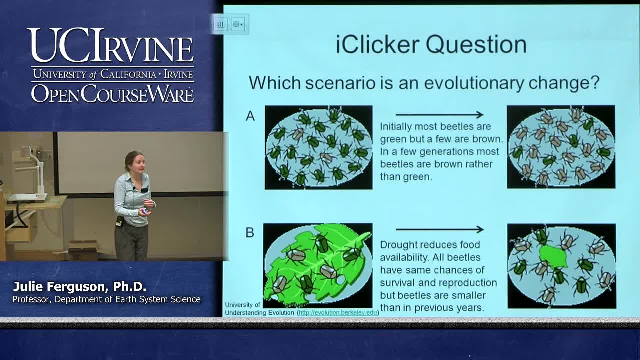 And so they may get smaller because they can grow less, But if we increase the food availability again, then they could get bigger. There's no real genetic change going on there, Whereas at the top what we're seeing is a fundamental genetic change. 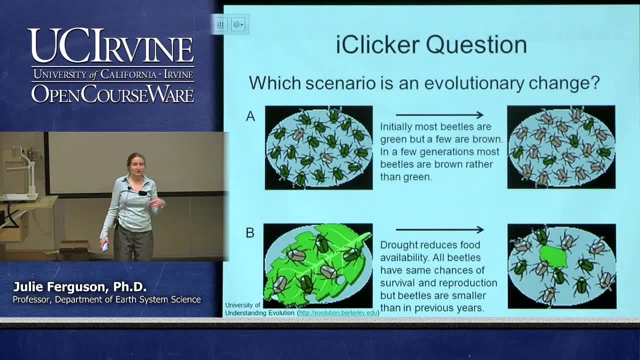 The genes that control whether those beetles are brown or green. the proportion of that is changing. Okay, so we have an evolutionary process going on And it could be that there is perhaps an advantage to being brown rather than green, Perhaps sort of some camouflage or something like that. 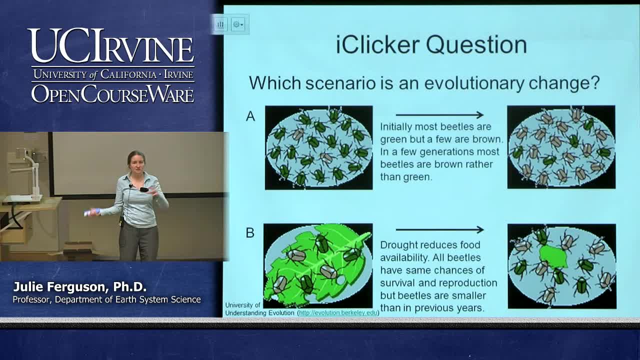 And so what we see is that there's a change in the genetic makeup of that population. Okay, And people are getting confused about this Because you're thinking about natural selection, which is what we're going to come on to next. But with natural selection, what we need there to be is some control that there's an evolutionary advantage to your particular mutation. 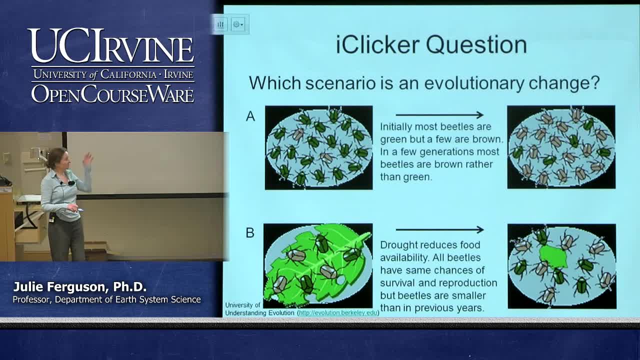 So we'll come on to that in a second. In general, if you find any of this stuff confusing, there's a really amazing website which I stole these diagrams from- which is a UC Berkeley, but they're pretty good- And it's called Understanding Evolution. 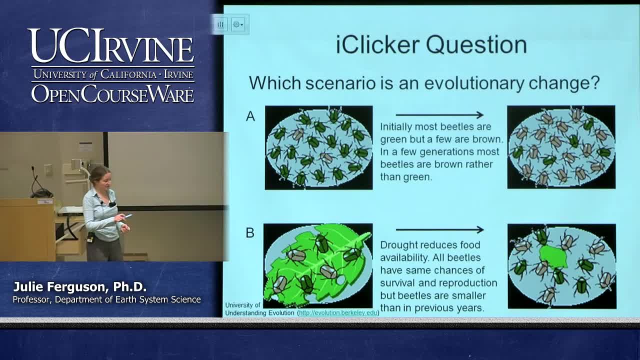 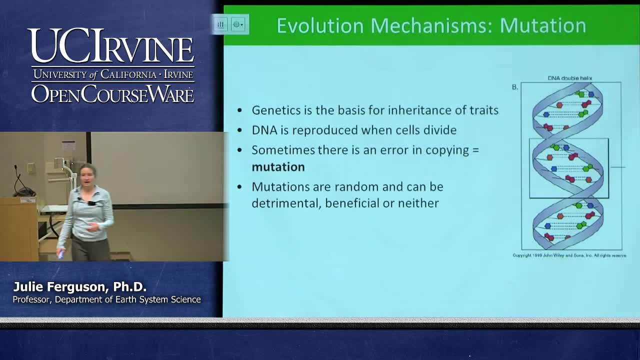 And they have lots of information And there's lots of little pages that describe some of the stuff we're doing today. So I do recommend you go and take a look at that if any of this is confusing. So let's think about our evolutionary mechanisms. 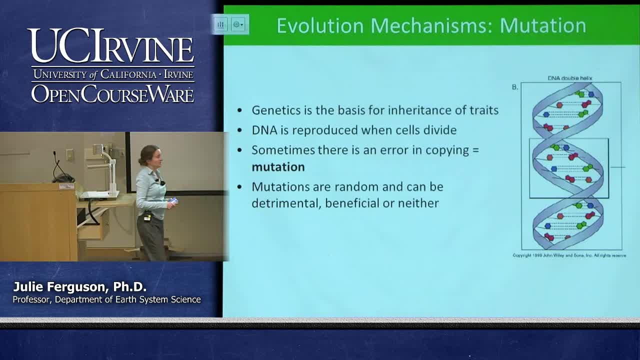 So what is it that creates changes in the genetic frequency or the frequency of certain genes in our population through time? So, first of all, we need to create genetic diversity. We need to have something different, And a lot of that happens through mutation. 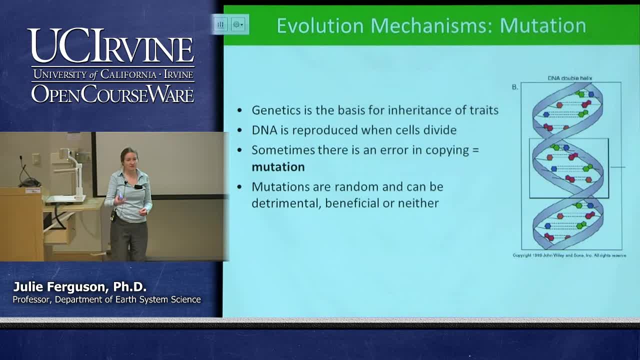 Okay, So genetics. is this basis for the inheritance of traits, because the genetic sort of code of the parent is passed on to the offspring, And DNA, our little double helix here after sort of created or not created by, but discovered by Watson and Crick at the pub. 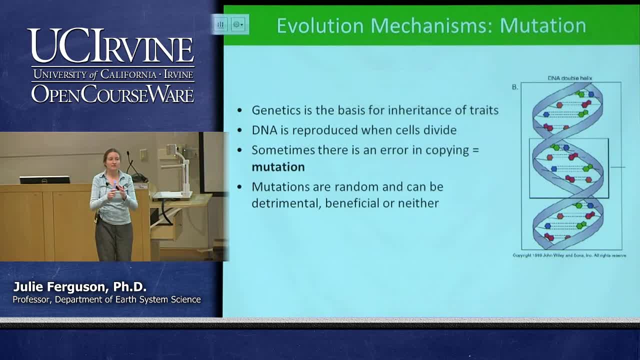 that sort of DNA gets reproduced. It gets copied whenever a cell divides. So whenever our cells divide, sort of when you're sort of healing and things like that, then that DNA is copied And through time little errors are made. It's what creates our aging process. 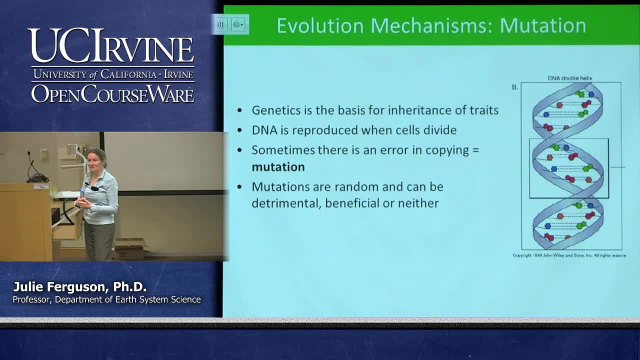 It's why I look a lot older than the rest of you, because my cells have copied a lot more often and little errors have been made. And a significant error in this sort of, in this copying process can cause a mutation, And mutations can be bad. 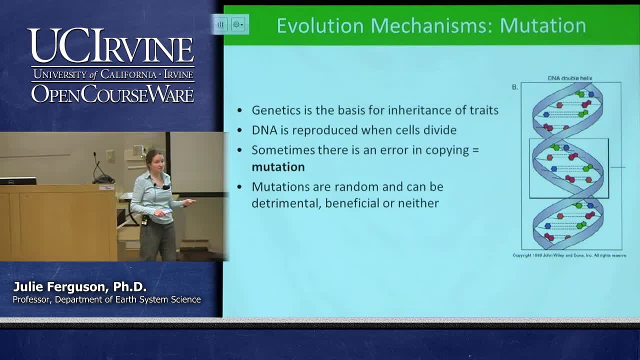 They can be detrimental for that organism. They can be beneficial, So they may give that organism an advantage. Or they can be just complete, They can be completely neutral, They can just exist, And so the key thing about mutations is that they're random. 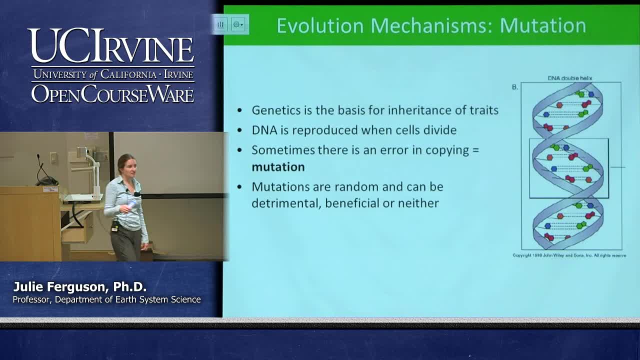 They don't occur in response to an environmental change. It's not that it got colder and so a mutation will happen to allow that. organism Mutations are happening all the time and they're random. It's just that some of those mutations might result in an organism that is better able to survive. 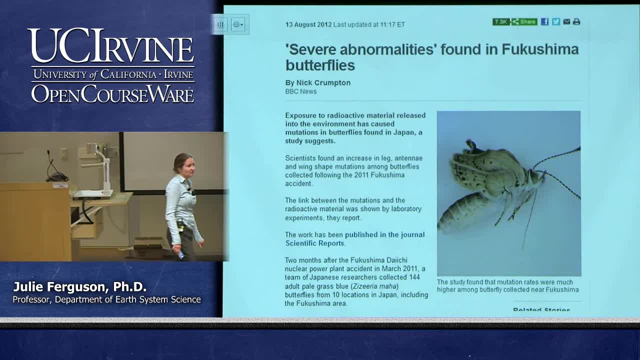 And, in particular, if you ever read comic books. we all know that radioactivity can cause mutations. right, But we don't get Spider-Man or anything else like that. But high enough radioactivity can cause damage to DNA And so when that replicates, it can cause mutations. 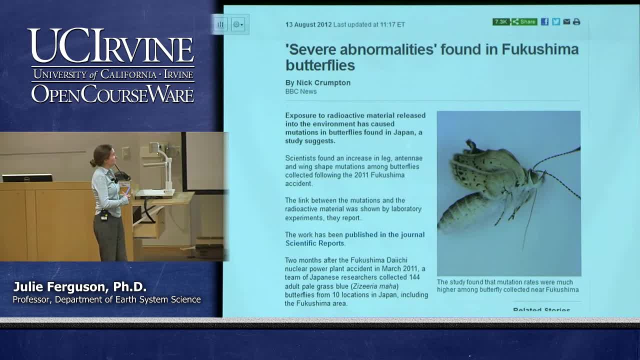 And, in particular, given that we'd already talked about Fukushima, I wanted to show you this, which is that, around Fukushima, that release of a very radioactive material did damage to the DNA of some of the organisms there, And so we did see these. 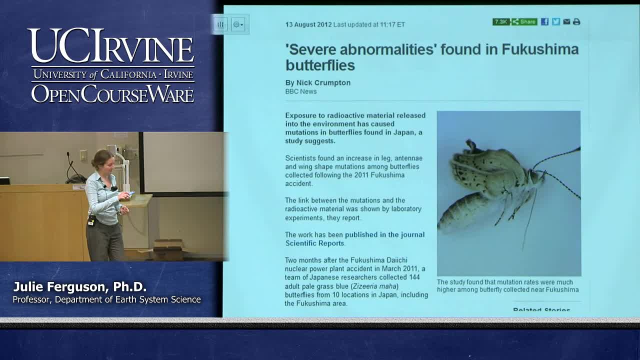 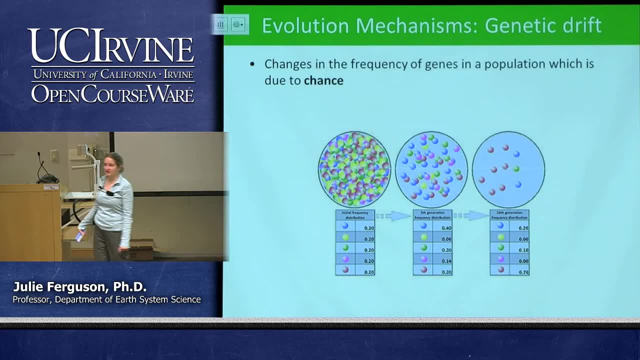 There's really weird mutations in butterflies and insects around there and probably still are Okay. So once we have our mutation, once we have our genetic diversity, there's a couple of different ways that we can shift the frequency of those particular genes in a population. 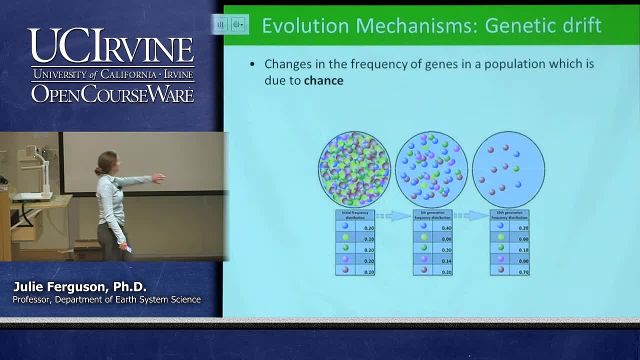 And the first of all is just by chance. So if I have a whole bunch of individuals, perhaps with different genetic populations, genetic frequencies represented by those different, different colors, if we just happen to kill off a lot of the population, then by chance we might end up with different frequencies of genes in our population. 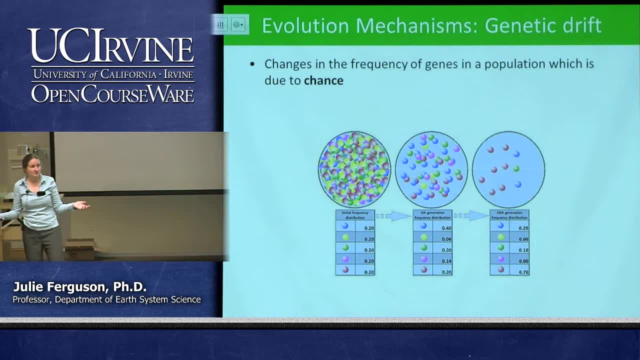 Not because of any particular advantage or disadvantage, but just by chance. So if you can reduce your population enough, then you're going to reduce your genetic diversity, And this has happened with elephant seals off the coast here. The elephant seals were hunted and their numbers got down to maybe as few as 10.. 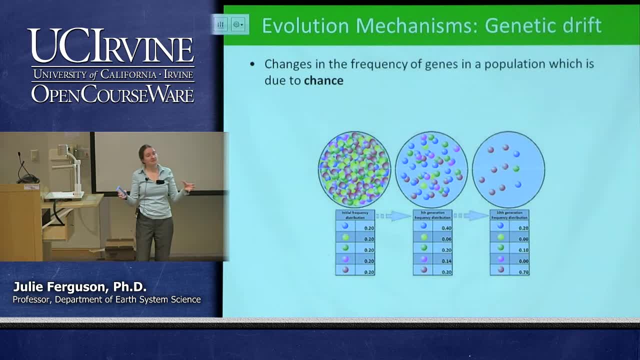 And now their population has grown again. but there's a lot less genetic diversity in that population, And so they're much more susceptible perhaps to change or to disease, because we don't have that diversity there. So just by chance we can end up with different frequencies of genes in our populations. 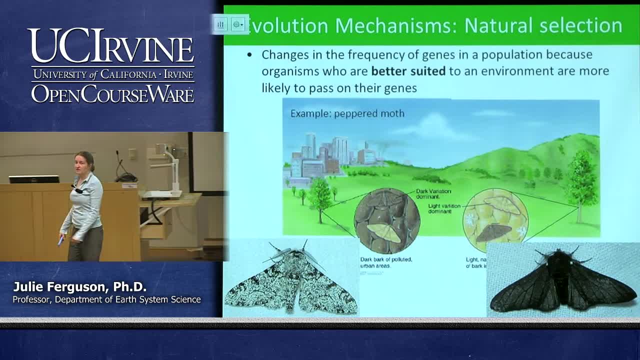 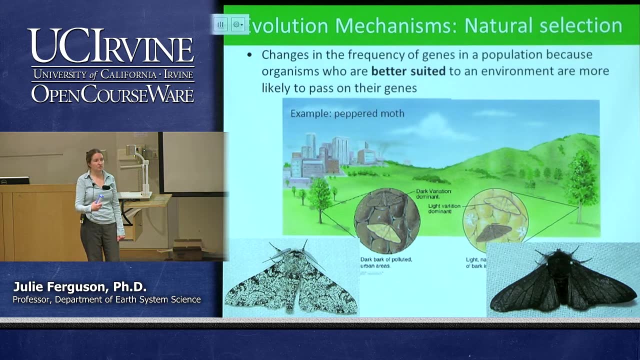 And then this is the one that people are more familiar with. This is the process of natural selection, And in this case we get changes in the frequency of those genes, not just by chance, but because those specific genes give that organism a slightly better chance of survival and reproducing. 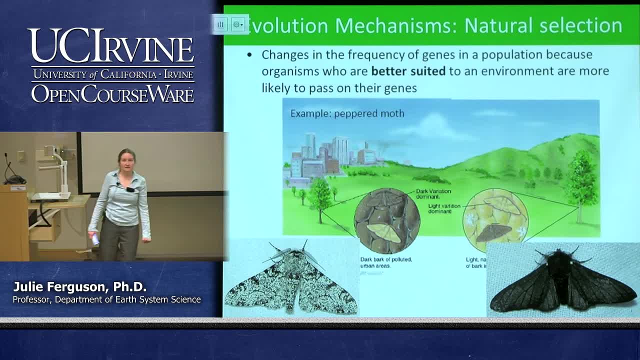 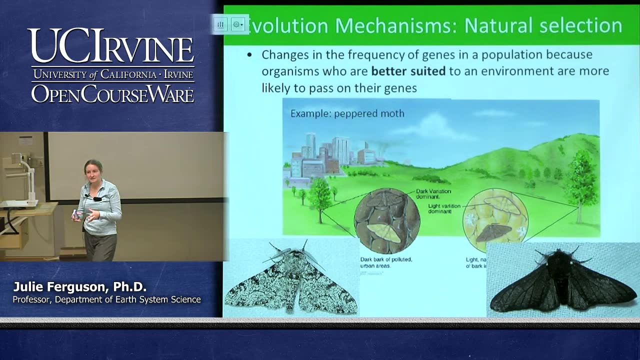 And so here's our classic example of something that has happened relatively quickly on human timescales, which is, we have our peppered moths And we have light-colored peppered moths and we have very dark-colored peppered moths, And when we had the development of cities, and especially around Europe, 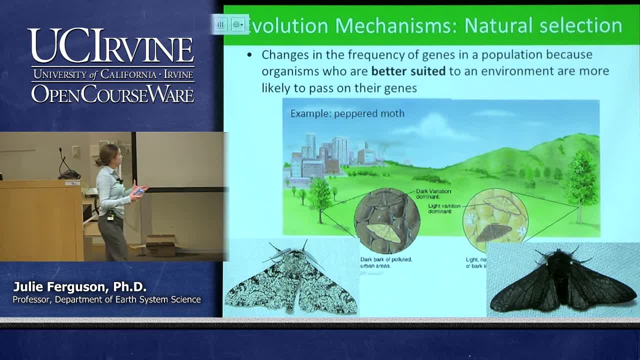 when we had, Yeah, so, lots of coal power and generating lots and lots of soot, then that could change the colours of the building, colours of the environment, And so the dark moths that were more camouflaged did better, And so we ended up with more dark moths, perhaps in polluted urban areas. 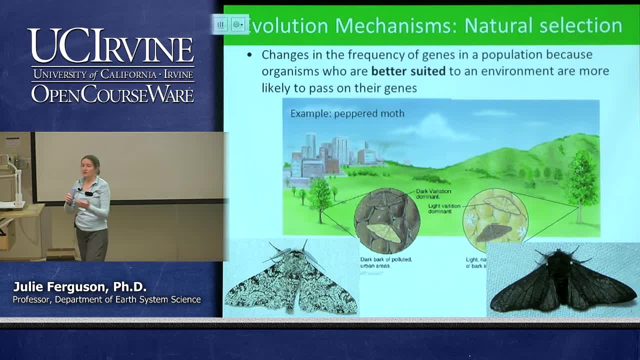 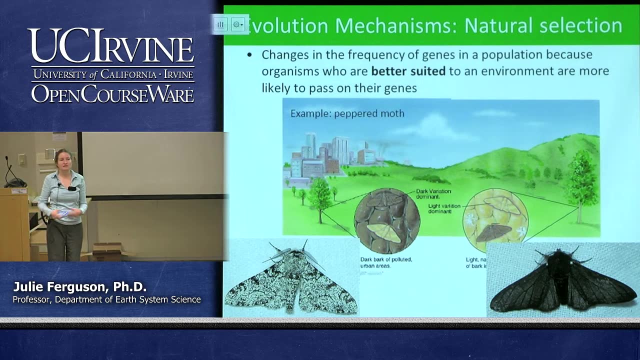 and more light moths in unpolluted areas where they would stand out against the environment, And in this case the different mutations here are giving something a bit of an edge. They're giving that organism a bit more suitability to the environment, And so one of the things that is a common misconception is that life is better today than it was in the past. 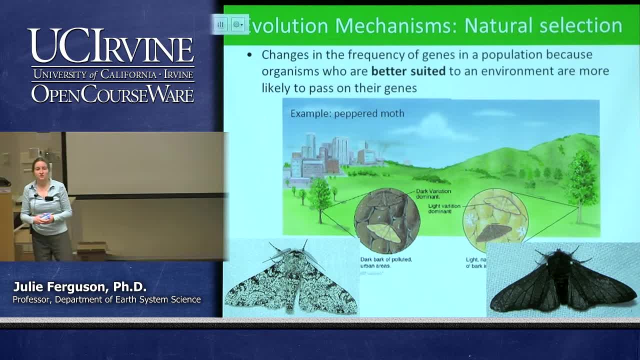 It's not better, it's just different. It might be better suited to environment, but that environment might change. It's not necessarily better, It's more complex. It's more complex perhaps, but that's it. So, in order for our natural selection to take place, 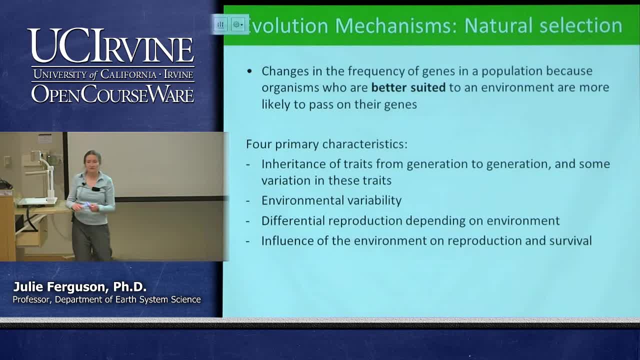 we need four fundamental things that we've mostly talked about already. We need the fact that we inherit traits, So a mutation is no good if it's not inherited by your offspring. if you're not going to give your offspring the same chance of survival. 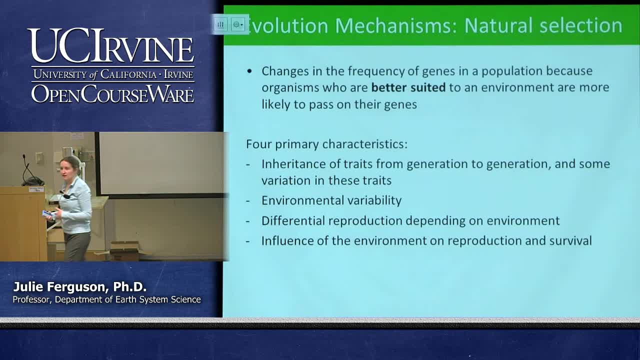 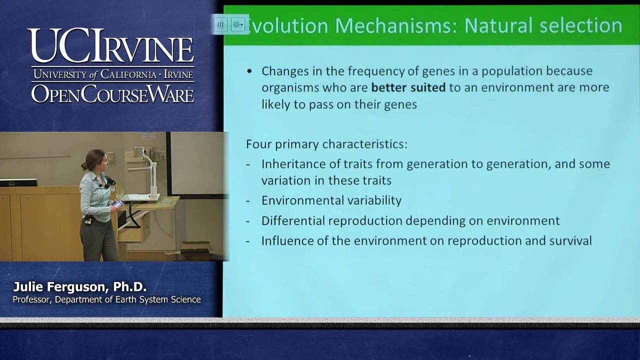 We need some sort of environmental variability, And that environmental ability, coupled with the success with that organism, means that we're going to have differential rates of reproduction. So those dark moths hang around longer, so they're more likely to reproduce, And so we'll get more and more dark moths in these polluted areas compared to our rural areas. 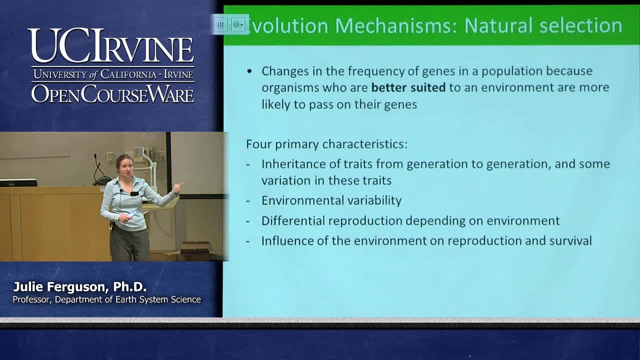 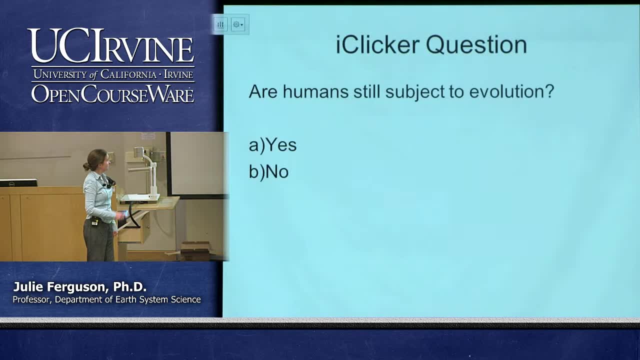 So this is our natural selection process. So we have chance and we have natural selection, And both of those can introduce evolutionary changes. So here's a question for you: Are humans still subject to evolution? Do we still undergo the process of natural selection? 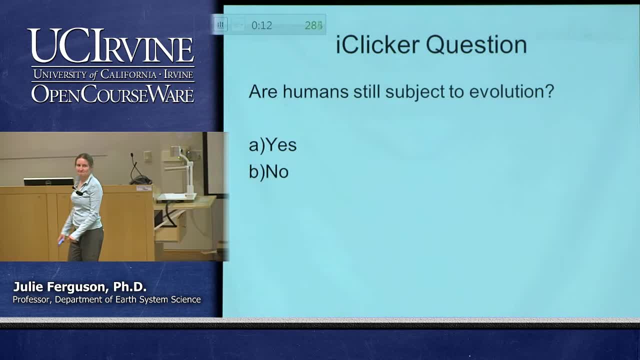 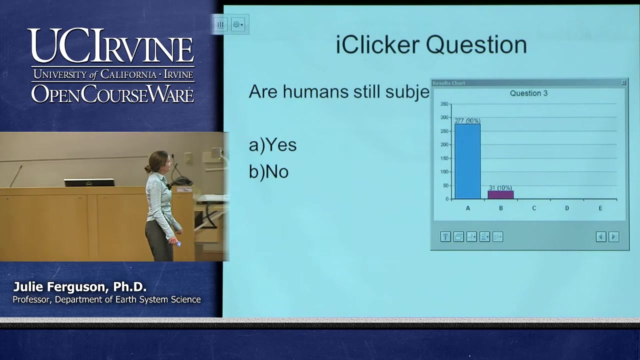 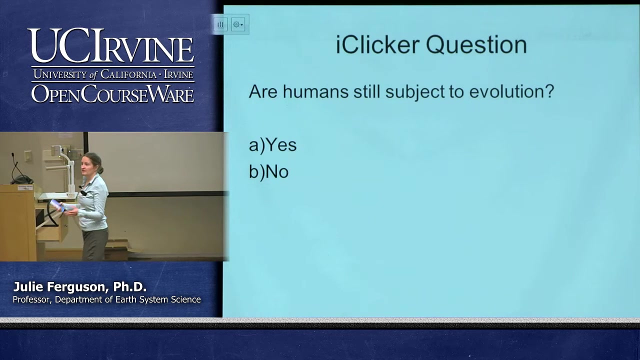 What do you think Last couple of seconds? Okay, So 90% of people say yes, 10% said no. So we've got a much better split this time and the 90% would be right. okay, Because we're constantly. our genetic code will be mutating, just like before. 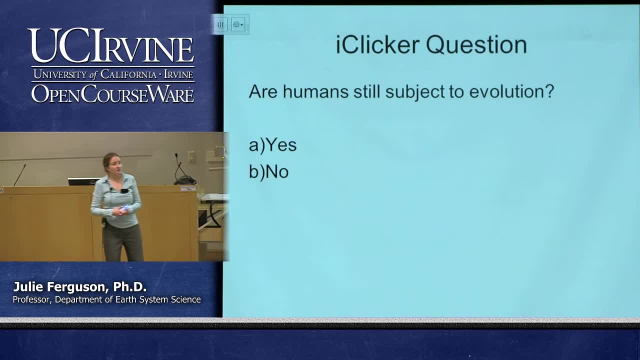 And there might be chance changes in our variation, But also there are certain changes that make us better suited and more likely to survive and reproduce. Can anyone think of evolutionary changes that might be happening today or in the recent past- And by recent I mean a few thousand years, because I'm a geologist- 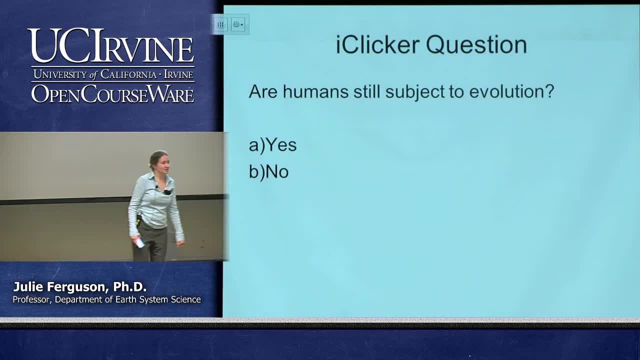 Yeah, Average height, Height definitely is changing. I'm not entirely certain. I'm not entirely certain. I'm not entirely certain. Is that a genetic change, or whether that's so we're better fed? I'm not sure. I'll have to look that up, but it's an interesting idea. 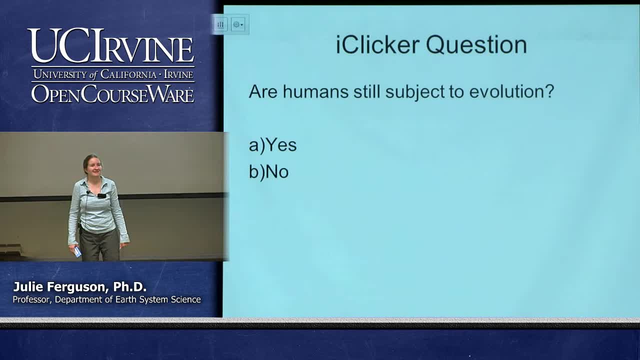 Yes, So definitely, we got anatomically modern humans 120,000 years ago, But we are still seeing some evolutionary changes, So our genetic material is sort of altering slightly. So, for example, things like lactose tolerance. Okay, so you can imagine how that might give you an evolutionary advantage, if you're able. 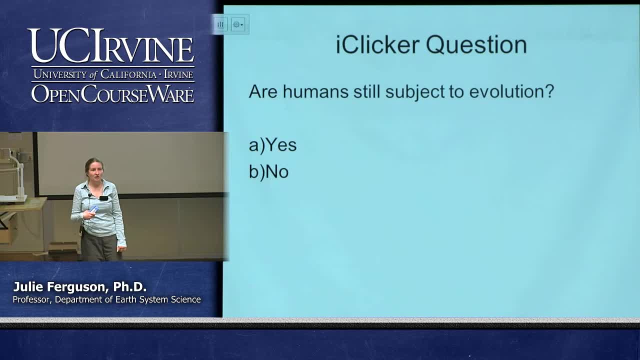 to sort of drink milk and sort of tolerate lactose for longer, then you're probably going to be able to have some higher calcium intake, And so what we see is that in areas where dairying started earlier on, a few thousand years ago, we have populations with higher proportions. 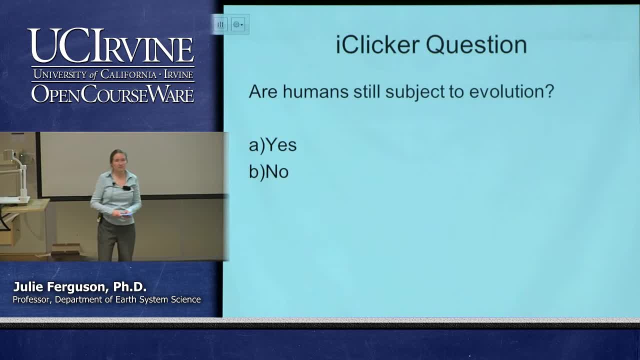 of lactose tolerance than in other areas. How many blue-eyed people do we have in the room? Wave at me? Hello everyone. We all share a common ancestor. okay, Blue eyes sort of happen, because one guy that lived near the Black Sea 10,000 years ago. 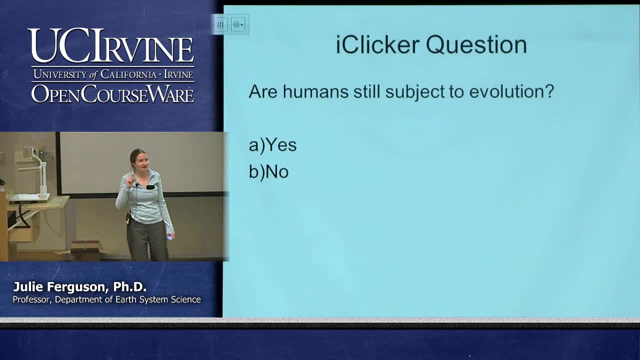 happened to evolve the genes for blue eyes, So before then everyone had brown eyes, And blue eyes is a lack of pigment in your eyes that makes them look paler. okay, And we're not entirely certain why that gave us an evolutionary advantage in sort. 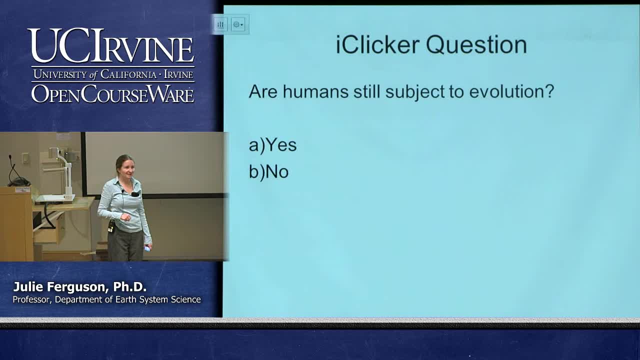 of northern Europe where that happened And where the most of the blue-eyed population is today. but it is recessive, so it is sort of tending to fade away. And not only that, but things like disease tolerance. so we're seeing more people. 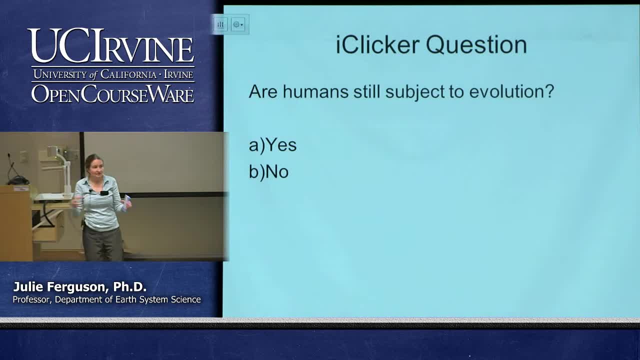 that are perhaps becoming immune to malaria. So living in cities has really forced us to develop immunity to certain diseases. So there's definitely changes happening all the time in our population. We're seeing changes in the frequency of our genes, So we're definitely still evolving. 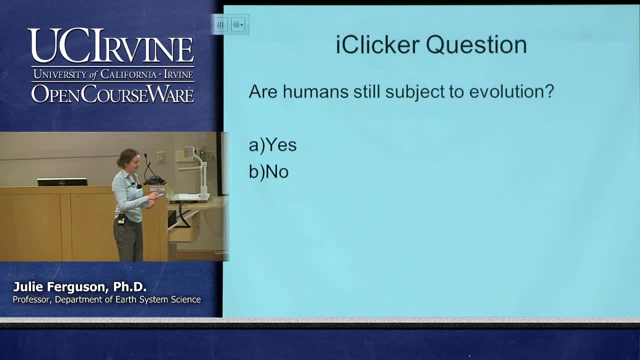 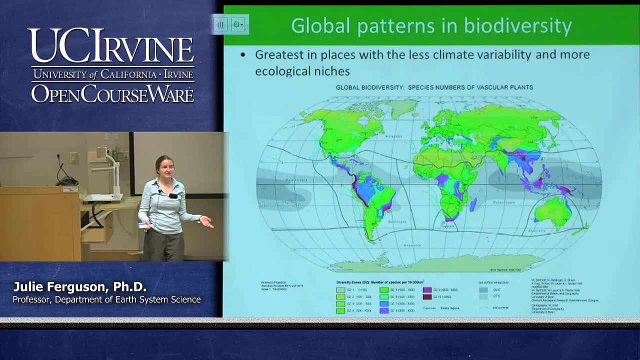 And natural selection. It might not work exactly the same as it did in the past, but somewhat still the same today. So if we add up all of our biodiversity, let's look at where that biodiversity is on Earth, And there's certain patterns. 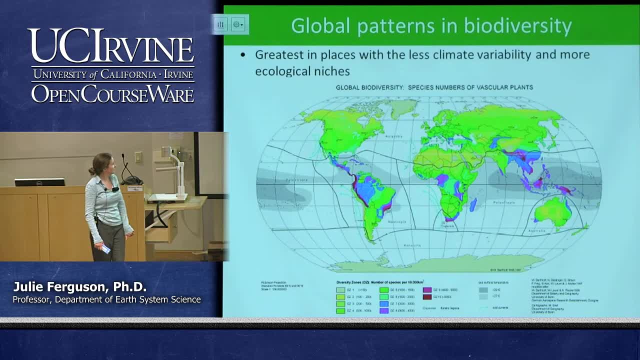 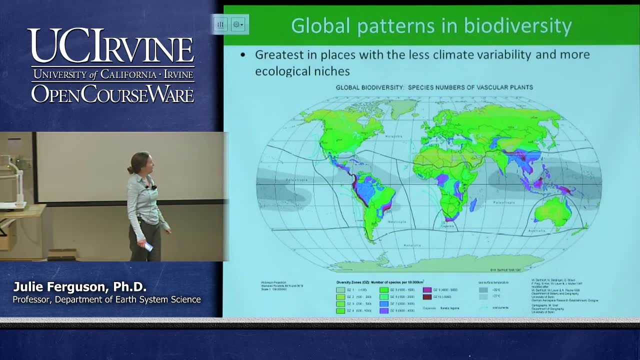 So my map here: the paler, the color, so sort of the creams and the yellows and the pale greens, where there isn't as much biological diversity, Those darker colors, the purples, blues and reds, are where we have a lot of biological diversity. 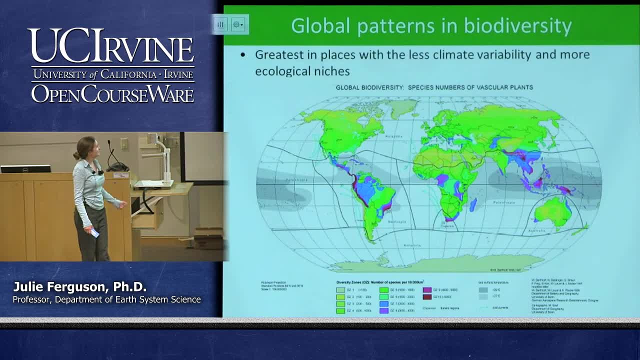 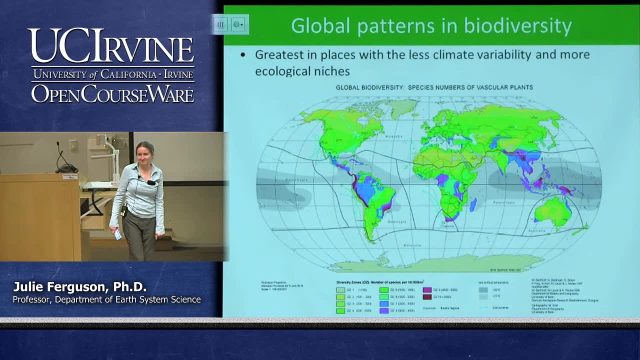 And what's the most important thing? What's the most important thing, What's the most obvious pattern that you tend to see? Where is the lowest diversity? The poles, absolutely. And the poles probably have lower diversity because we see it's a more extreme environment. okay, 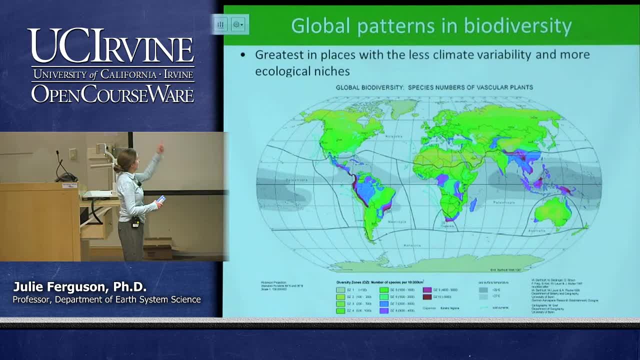 And also we see a lot more changes there through time, whereas actually around the tropics, even where we see perhaps our glacial, interglacial cycles, our ice ages, we don't see as great changes there as we do elsewhere, And so what we've had is we've had a lot less climate variability. 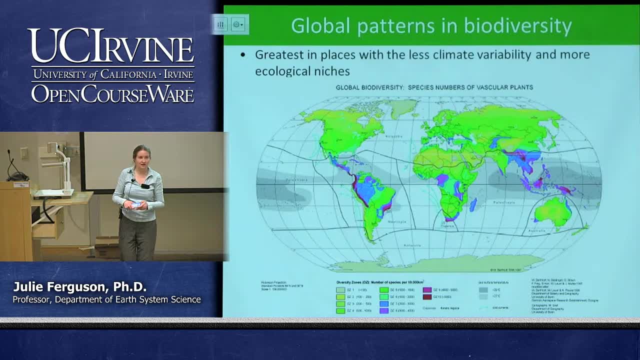 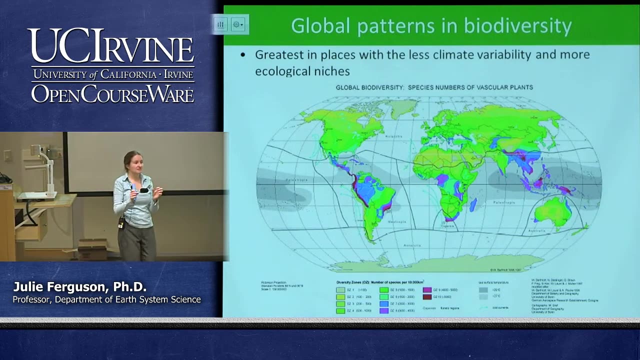 And we have a lot more ecological niches in certain places as well. So around South America, for example, we have big mountain ranges and that can isolate populations and create these different ecological niches which allow different species to exist. Just remember, we said that if two species existed and they had exactly the same requirements, 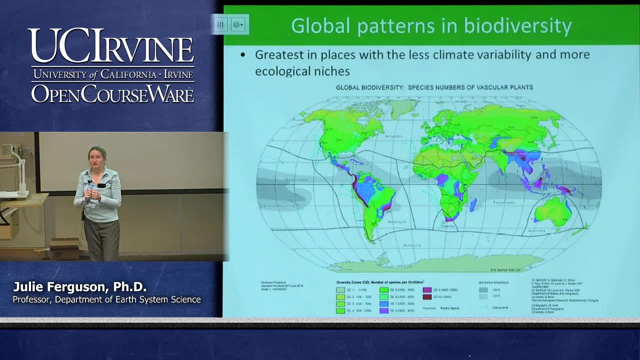 in a location, then one would outgrow the other. So that's what we're trying to do: We're trying to out-compete the other. But if one of them is slightly better adapted to a certain ecological niche, then we can have those two different species living in the same place. 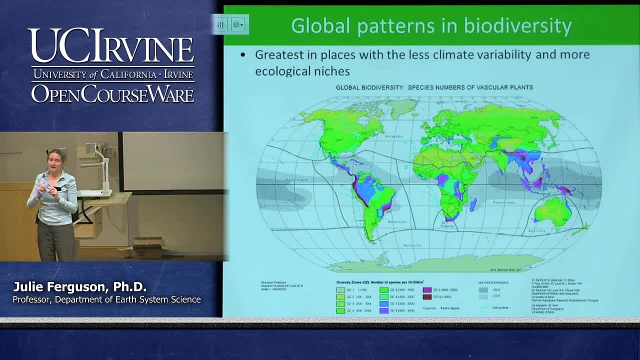 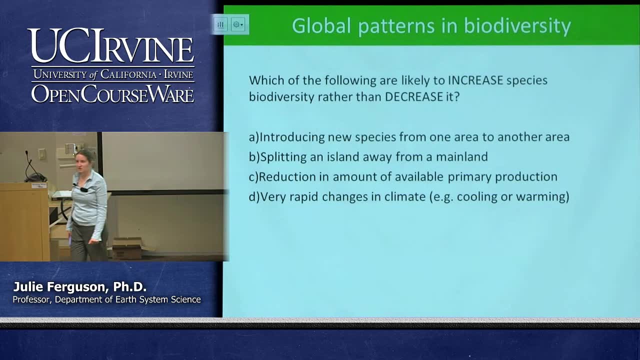 So if we have enough ecological niches, enough variation in our natural environment, then we can create biodiversity, okay. So my question for you is: which of these four things is likely to increase species diversity? So increase the number of species rather than decrease the number of species. 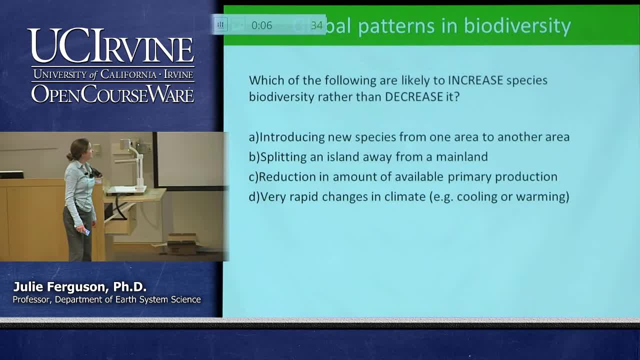 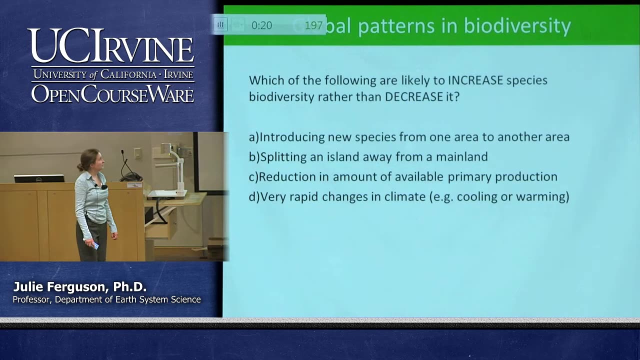 So would it be? introducing a new species from one area to the next, Splitting an island away from the mainland, A reduction in the amount of available primary production, Or very rapid changes in climate? Which of those do you think would increase species diversity? 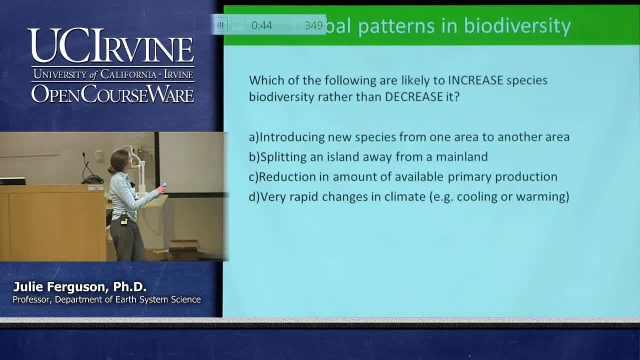 I think we have most votes now, so let's take a look. So most people said A, So we have a lot of votes. So we have a lot of votes. Okay, What's happened when we, as humans, have introduced new species around the world? 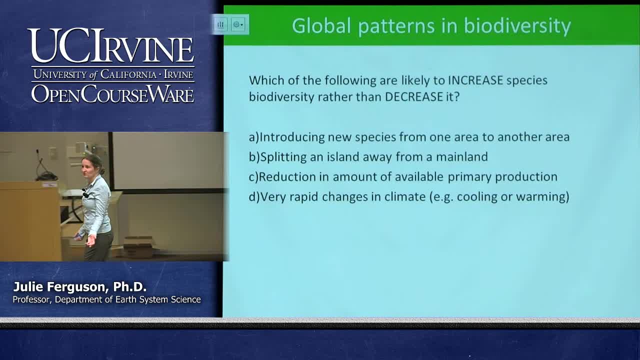 Have we increased species biodiversity? What have we done? We've killed off a lot of things. So, for example, if we've introduced rats to a certain area, okay. So if we rule out A, would you like to vote again? 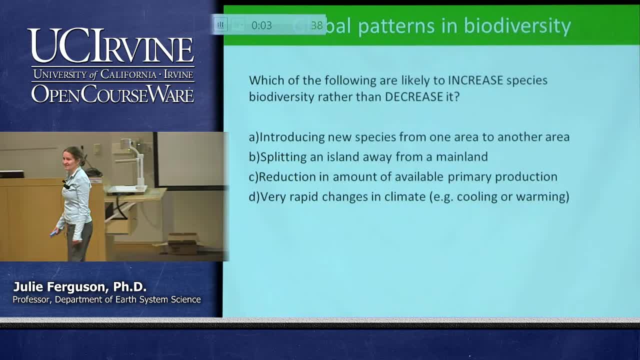 Okay, So think again. So if A isn't the answer, so remember, if we introduce two species and they have the same number of species and they have the same number of names of needs, then one is always going to out-compete the other. 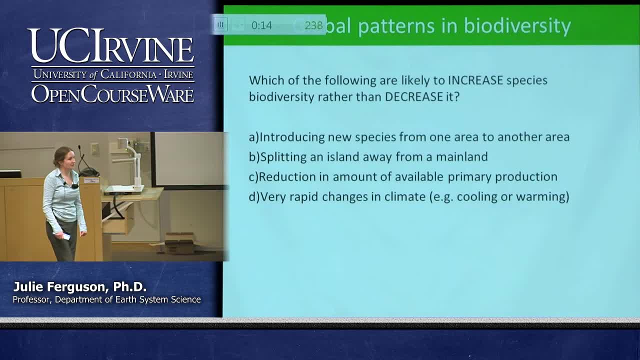 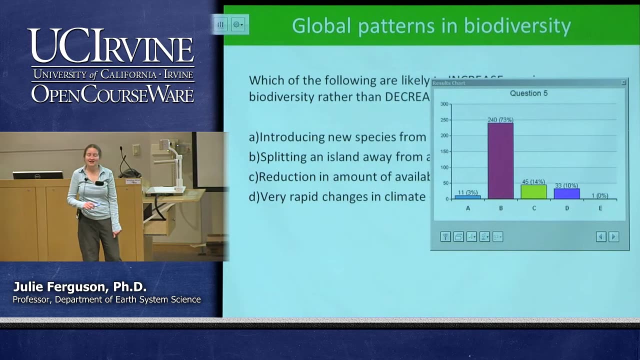 So if we're going to introduce lots of different species together, we're going to decrease biodiversity. Last couple of seconds. Let's take a look this time. So 11 people are still sticking with A, but the rest of us have mostly shifted to B and B would be correct. Okay. So what you're doing there is you're creating different populations. So, for example, if an island is split away from the mainland today and we previously had a population of animals, then what we have is we have distance between them. 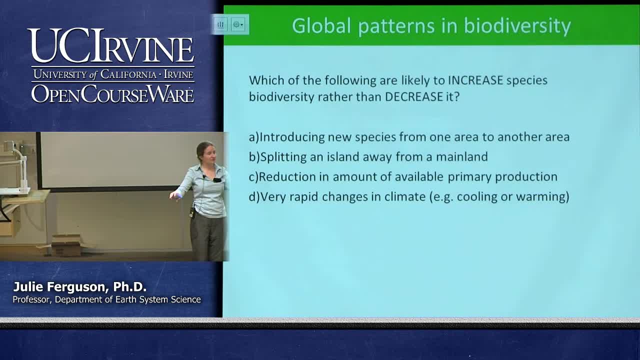 They can no longer interbreed as populations. So we have two distinct populations, and what might happen is that there might be slightly different environments on the mainland versus the island, And so, if we give it enough time, then they could evolve into different species. If we have different natural selection processes going on or we just have different species, then we're going to have a different population. So genetic drift happening by chance, then we can create two different species. And if those species are far enough apart for long enough, 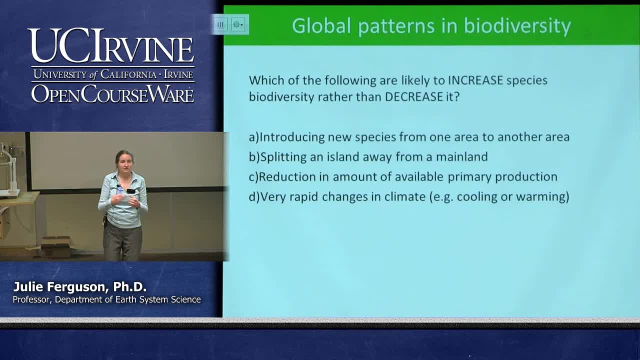 then, when they are reintroduced together, if there's been enough change, then they would not be able to reproduce, and so we'd have two different species again. So splitting an island away from the mainland is a really good way of creating new species. 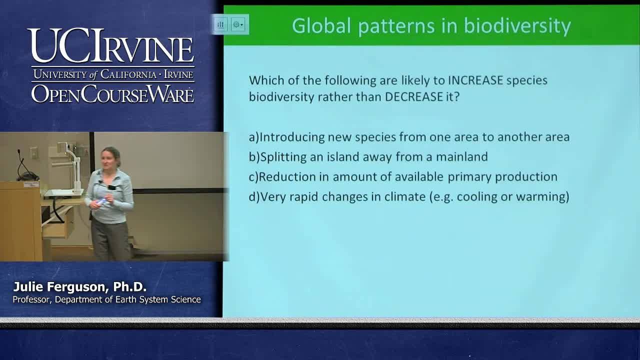 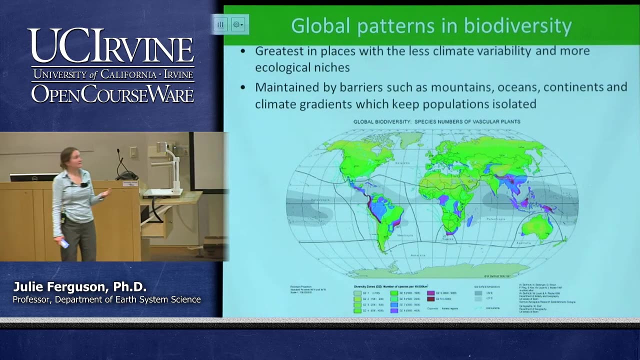 And so if you go to the Galapagos, the very famous Darwin's finches, where all of these little finches on different islands and have different adaptions, is a good way of looking at this. Okay, So our biodiversity is maintained by things like mountains. 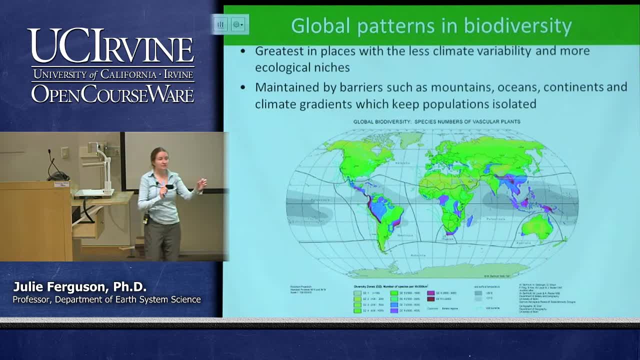 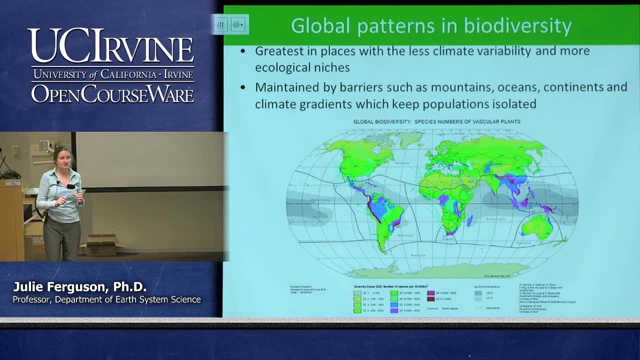 or oceans or climate gradients, things that keep populations isolated. Those isolated populations can change through time and we get different species. Okay, So things like our Andes mountain range in South America or things like the Sahara Mountains, and we get different species. 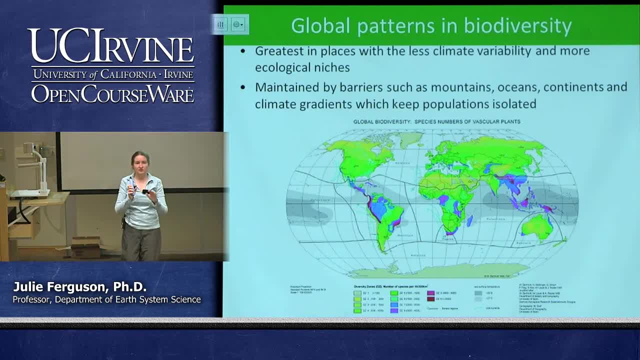 So if we were in the Sahara Desert, it would mean that you'd get different vegetation on either side, because we wouldn't be able to have plants that are expanding into the desert and passing that. So these things will change our biodiversity, And this is true deep in the geological past as well. 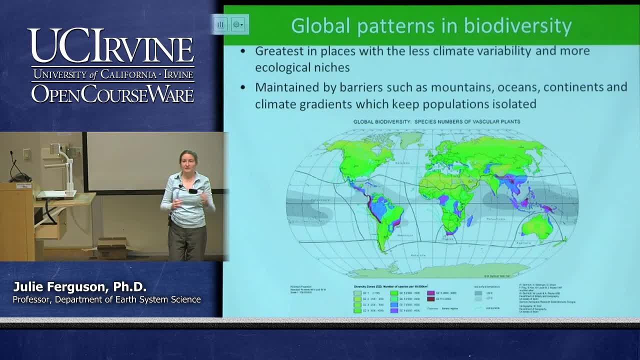 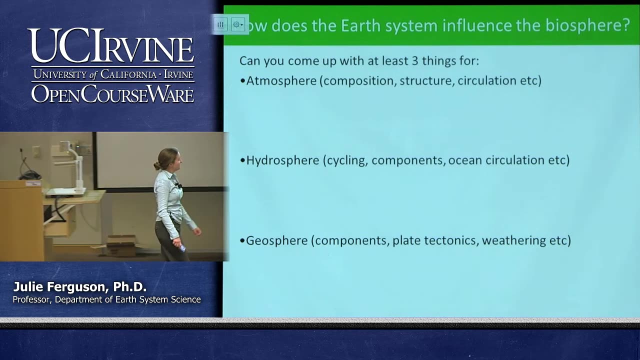 When we built our big supercontinents, then we brought lots of areas together, and so we saw changes in the biodiversity associated with that, because things could then compete and we saw reductions in biodiversity. So that was the things I wanted to cover today. 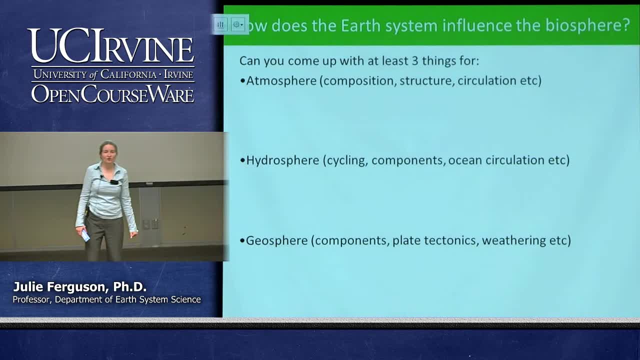 but I also wanted to give you a chance to start thinking about the concept map idea, that thing that most people have been ignoring because it's not week 10 yet. But I also wanted to give you a chance to work on it together with me. 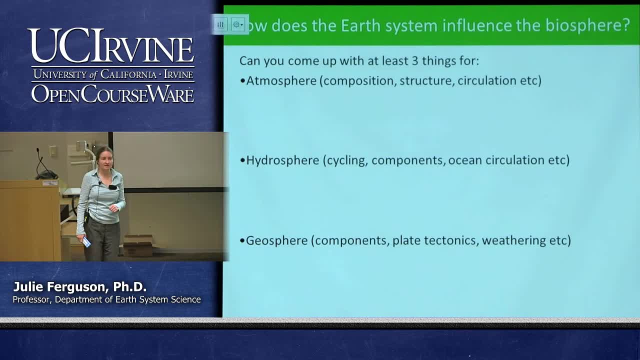 So we'll go through these and we'll spend a couple of, or maybe five minutes and then I'll give you some suggestions. But I want you to talk to the people around you and come up with at least three things for each of these. so how does the earth system affect the? 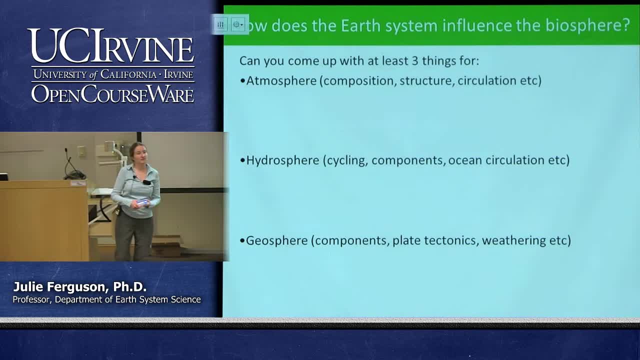 biosphere. so how does the atmosphere affect the biosphere? So you can think about the composition of the atmosphere, the circulation of the atmosphere. so things like our temperature, rainfall patterns, things like the atmospheric pressure, how might that affect the biosphere? 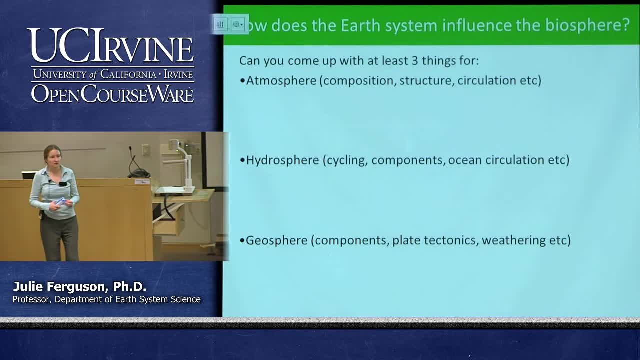 How would the hydrosphere affect the biosphere? So you can think of the different components of the hydrosphere, things like oceans or streams. how would that affect our biosphere? And then the geosphere. that one's more difficult. 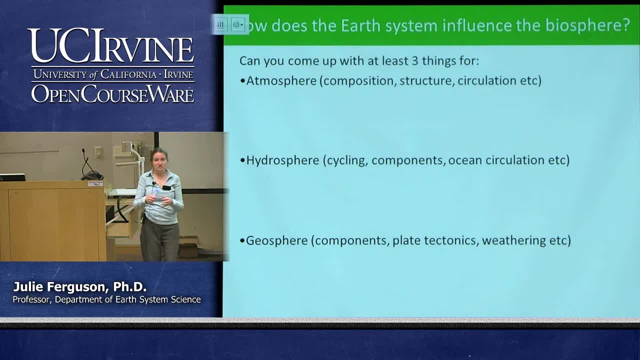 but I just gave you an example of how things like continent shifting position might change the habitats, or mountain ranges might help biodiversity. So see if you can talk with your neighbors and come up with at least three things for each of these, and this might give you a bit of a head start. 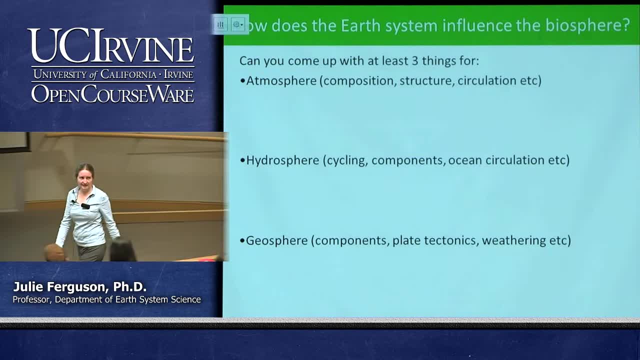 Right, so let's take a look. So I've been grilling the people on this side of the room, so let's see how the people on this side of the room are doing. I would like a suggestion. I'm going to give you a question. 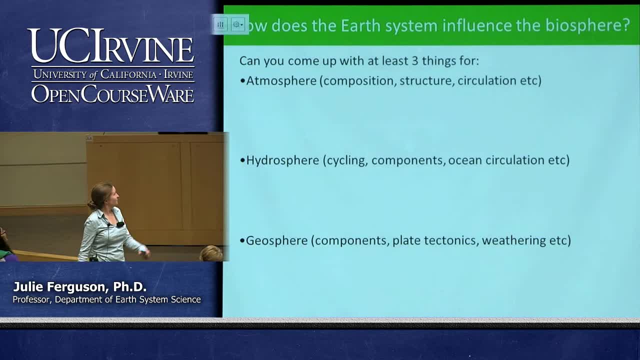 Suggestion for how the atmosphere influences the biosphere. Does anyone have suggestions for me? I'm sure you do have suggestions for me, You just have to be brave. Yes, So for circulation, the high and low pressures, so they can bring either like sunshine for photosynthesis. 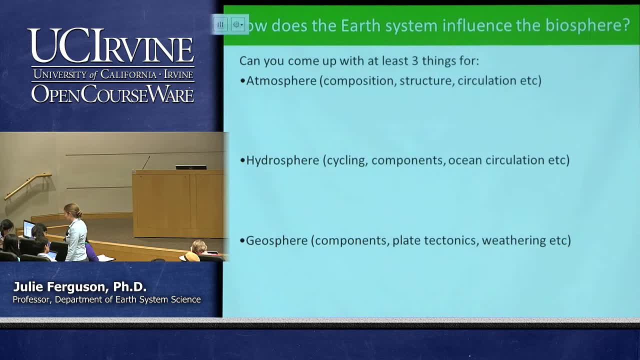 or rainfall, for more plant diversity? Absolutely So. things like our atmosphere, our atmospheric circulation is moving energy around, so it's affecting temperatures, which might affect what life can exist. It's also really affecting our precipitation patterns and that has a very strong control. 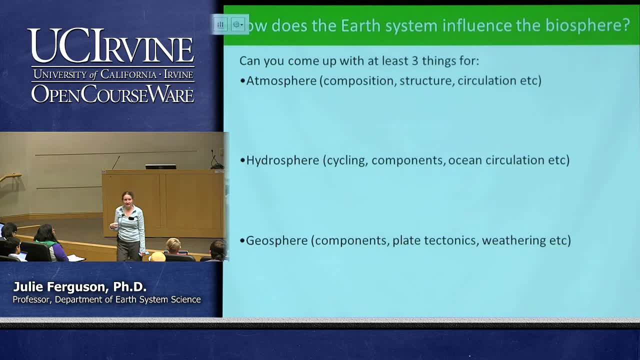 on where our different biomes grow. So definitely we have the atmospheric circulation plays a really important role. so our subtropical high pressure, where we have our deserts, versus things like our intertropical convergence zone at the equator where we have our tropical rainforests. 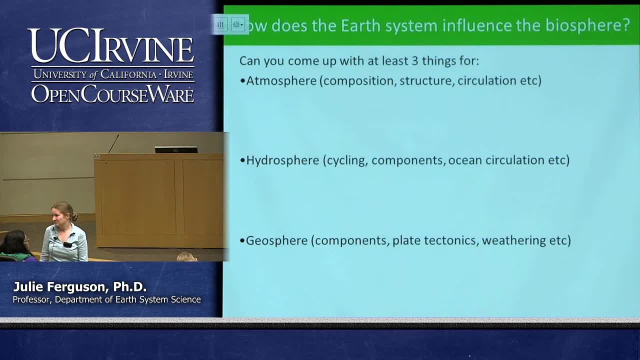 Does anyone have any suggestions? Anyone else have a suggestion for me? What does the atmosphere consist of that we quite like as humans? Oxygen, Oxygen, absolutely So the atmospheric composition. we have oxygen in our atmosphere which allows us to breathe. 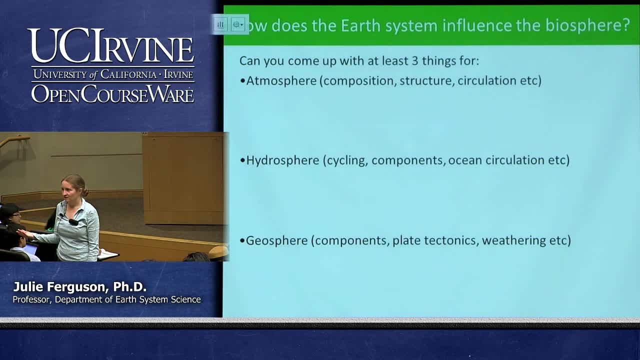 What else does it have in the atmosphere that plants might want? Carbon dioxide. So I heard nitrogen over here and they're right that there's lots of nitrogen in the atmosphere as well, and we're going to talk about that on Friday- how nitrogen can get fixed. 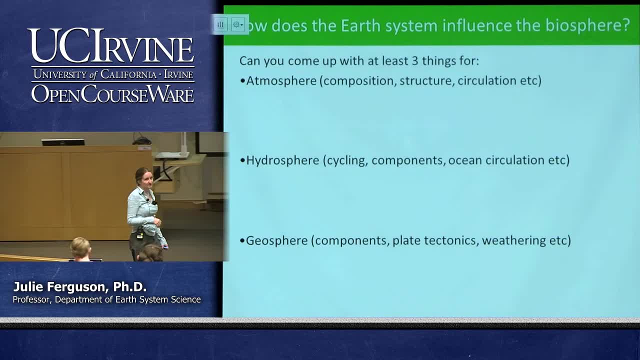 by things like lightning strikes from the atmosphere to the ground and that provides a certain amount of our nutrients. okay, Anything else for the atmosphere? I heard a really good one back there before. Why do we put on sunscreen UV? What's up there that life might quite like in the atmosphere? 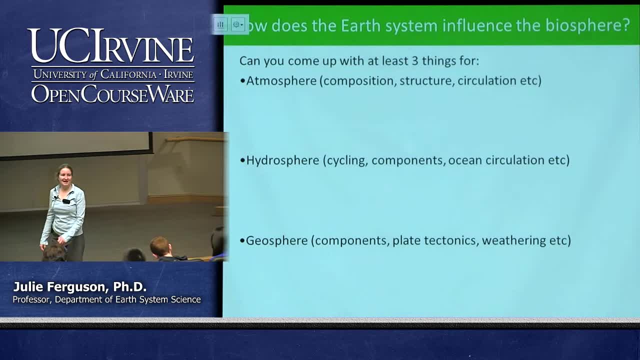 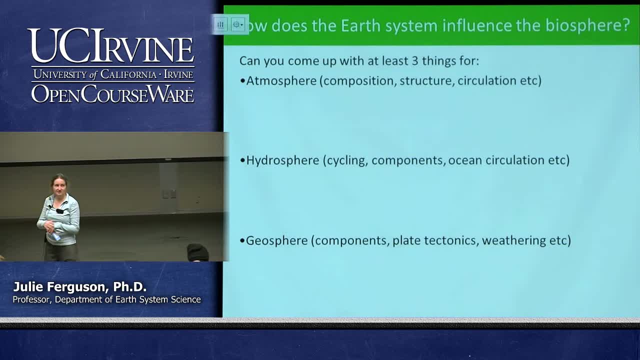 And it does also protect us from the ultraviolet damaging radiation that could cause mutations in our cells and make life pretty miserable on Earth. okay, So things like our ozone layer, which is again related to atmospheric composition. What else does the atmosphere carry? 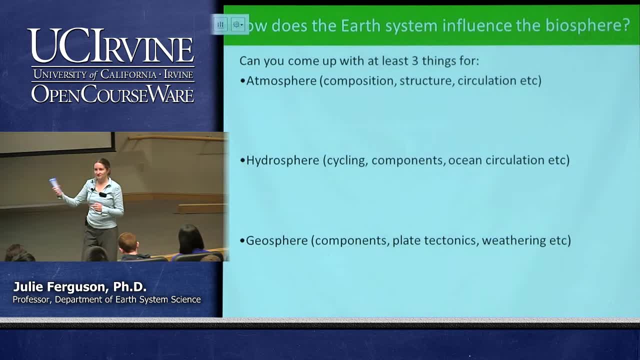 Water, Definitely water, and so we've sort of said that water is really important for life and definitely our atmospheric circulation controls the water, but also there's just lots of water in our atmosphere that we're not going to be able to control. 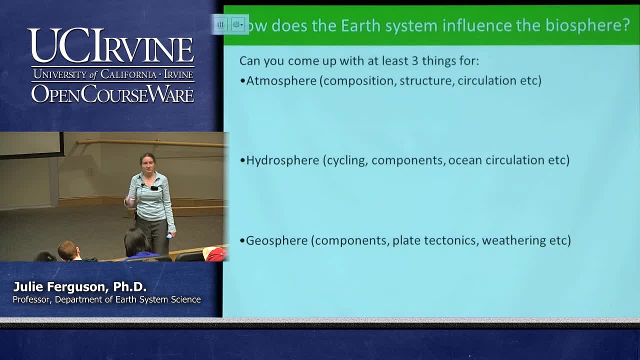 anyway, and we know how uncomfortable it gets and how much things dry out when the Santa Ana winds come through. so the presence of water vapor in our atmosphere helps. what else that is perhaps not a gas, but what else is carried by the atmosphere that is might be important for life, perhaps in the 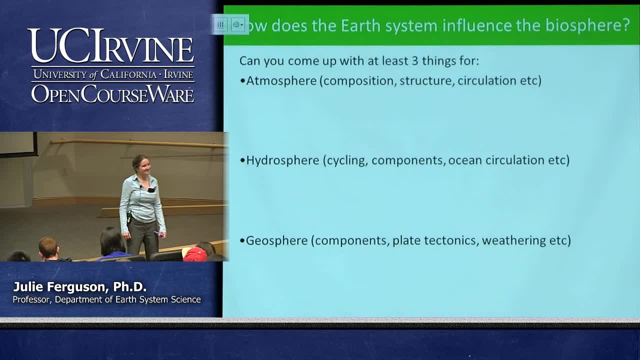 oceans, dust, okay, so remember we had things like aerosols, we had dust and things like the big dust storms that come off the Sahara Desert and so dump dust into the Atlantic there have a really strong effect on the nutrients availability in the surface ocean. so things like the atmospherics of movement 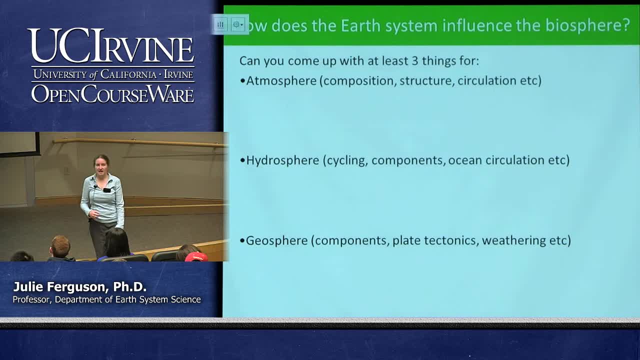 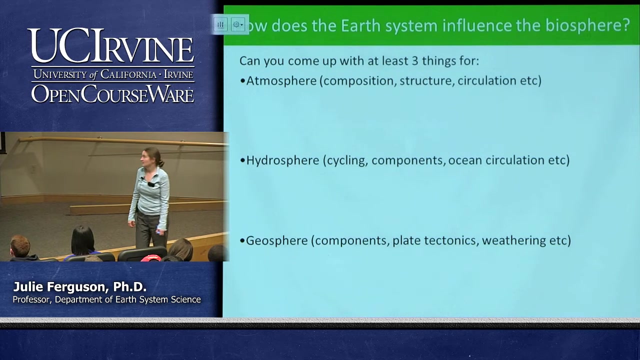 of dust around the material. what else does the atmosphere move? that might be very related to plants for those of us who have allergies: pollen, okay. so the atmosphere can also help the biosphere and distribute itself to new areas and transport new life to different places. you so? those are some of my suggestions. I'm going to list a few in a second which. 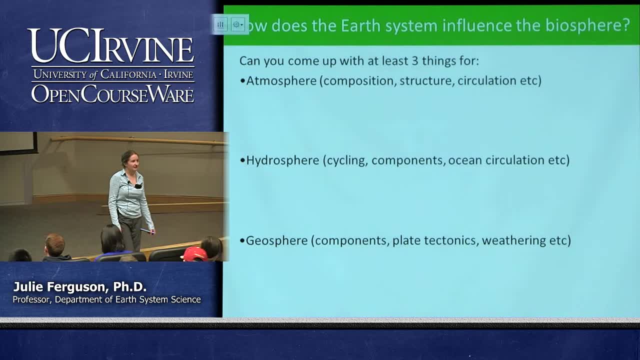 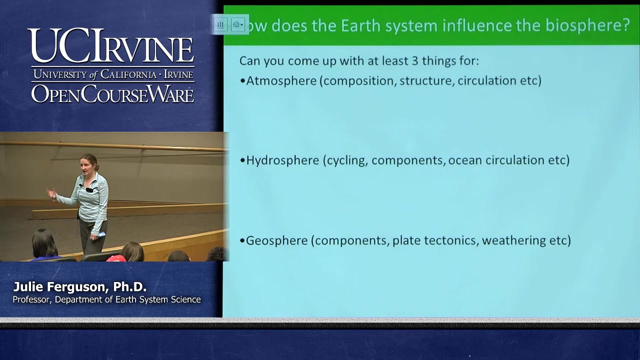 might or might not be those. how about the hydrosphere? how does the hydrosphere influence life on earth? rainfall: we definitely have rainfall going on, which we need for life. what else? yeah, cellular function, absolutely so. so the reason we need that water is that we need water in our cells for some of the chemistry. 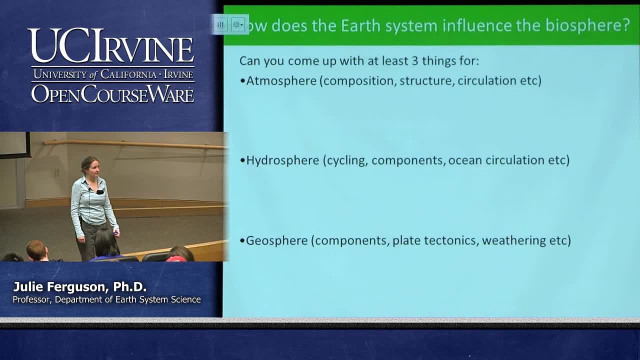 that allows us of metabolism to form. what does the, the hydrosphere consist of? what are some of the big reservoirs? oceans, yeah, and so the fact that the oceans are there provides a habitat for life, as does freshwater- different lakes and streams- provides habitat for life. what else does the hydrosphere do? what? 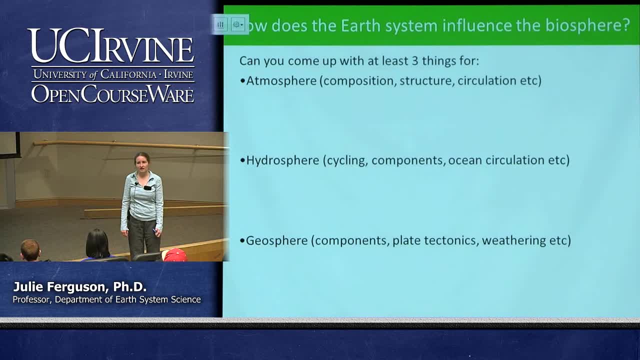 does the, what does streams carry? that might be important for life. that's just really important for everything that we're talking about now. we're talking about sediments and nutrients. so, for example, remember we talked about chemical weathering and so we get lots of nice dissolved stuff in our streams that goes down and goes into the oceans. I mean. 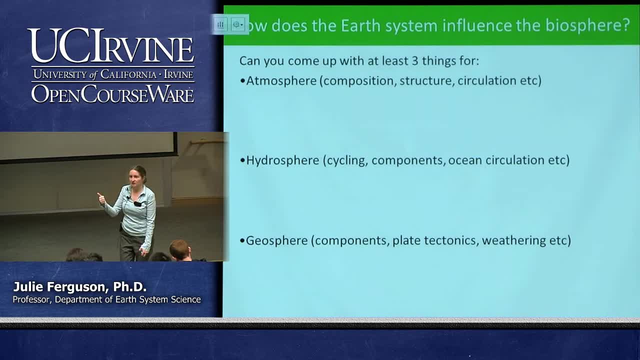 it creates our salinity, which creates different ecological niches, so there's our different habitats. but it also transports things like phosphorus and nitrogen that life needs. so we have the the hydrosphere bringing in nutrients. anything else for the hydrosphere? what did we? 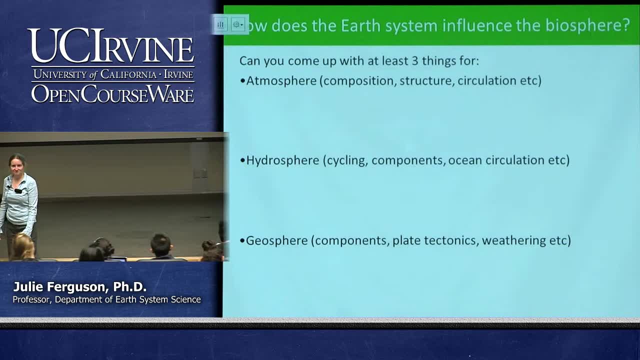 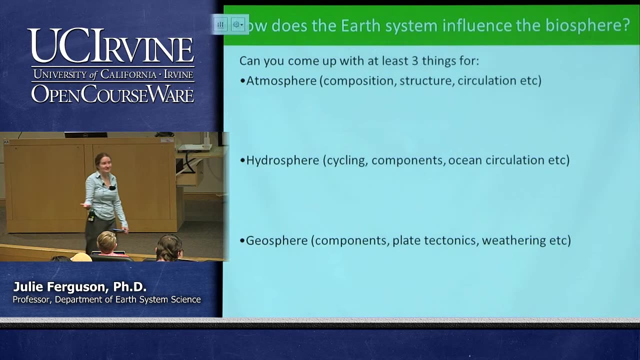 talk about that everyone hated doing for ocean circulation, sorry gyres and what else. what happens along the edges of continents? upwelling and downwelling. why was upwelling important? because it brings up nutrients. so again we're sort of thinking about how the oceans can survive. 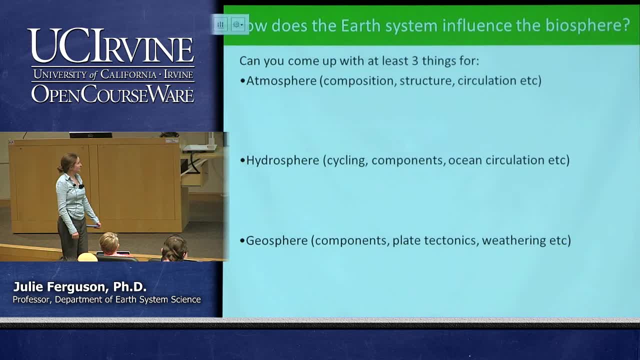 circulate and redistribute nutrients. I also had a really good comment at the back again is that the hydrosphere is another thing that helps create our climate and moderate our climate. it stores heat, it transports heat, so it affects local temperatures, which in turn affect our 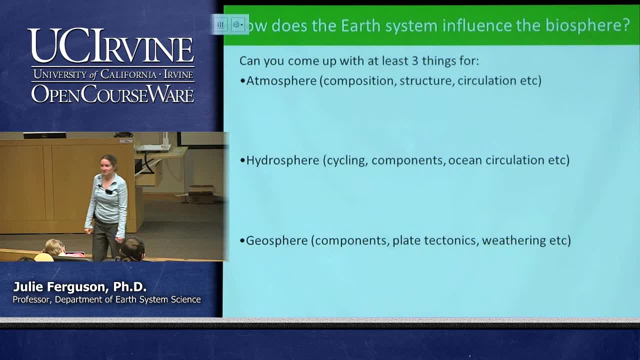 biosphere. and how about the geosphere? this one's a bit more challenging. does anyone have something for the geosphere? permeability and porosity, permeability and porosity, and so things like can life exist in those little spaces? that's definitely one. anything else? volcanoes: what do volcanoes do? yeah, they make new areas of land. so, again, the fact that 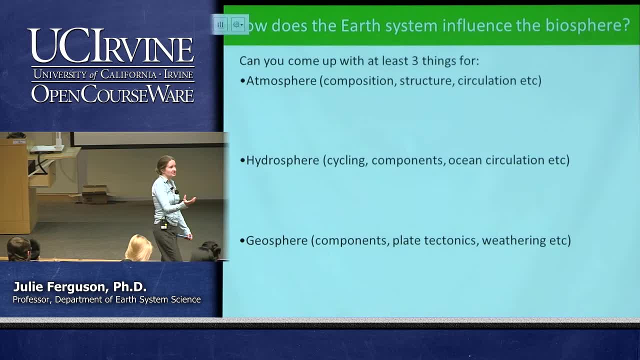 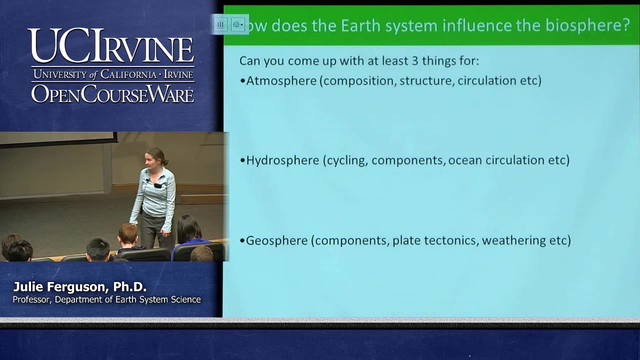 we have volcanic activity. tectonic activity is creating new land. what else can it do? would you want to be the biosphere next to a volcano? necessarily, it can also act to destroy the biosphere as well, in local patches. so volcanic activity can both create new habitat, but it also 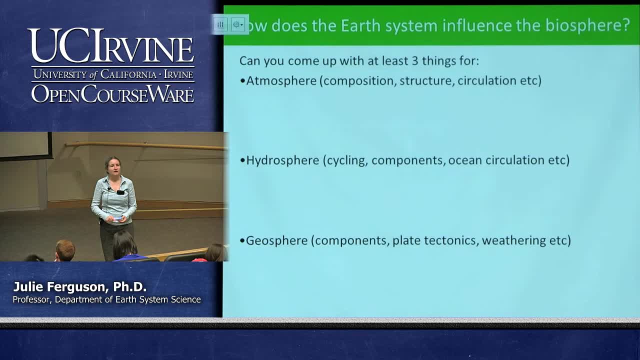 can destroy the biosphere. okay, yeah, okay. things like weathering. remember, chemical weathering is what gets things into solution, into our streams to go into the ocean in the first place. it creates our salinity and take tectonics. it moves our continents around so we can create mountain. 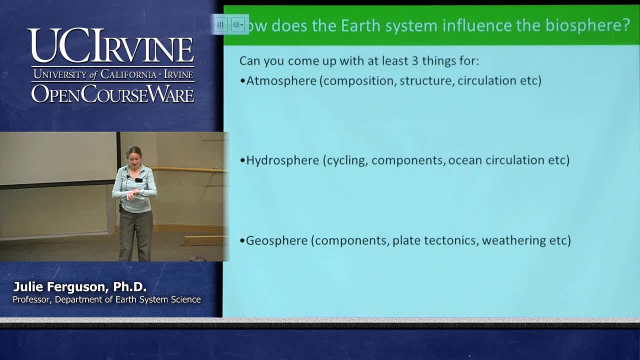 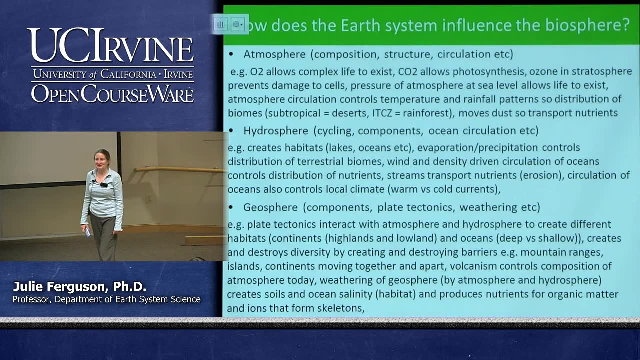 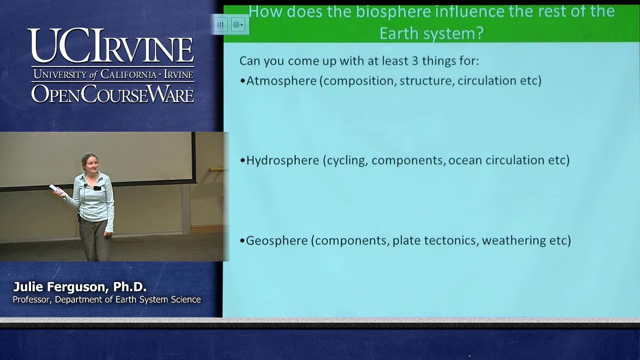 belts and we can create different amounts of biodiversity. everyone keeps packing up early. okay, so there's some of my suggestions, so I'm taking pity on you all and giving you some suggestions to start. not only that, I'm even nicer than that and I was going to ask you this, which is, in turn: how does the biosphere affect? 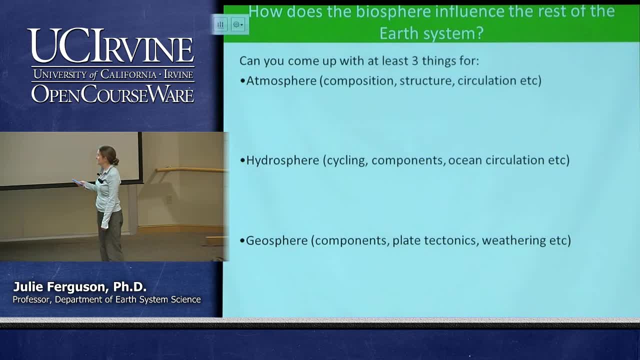 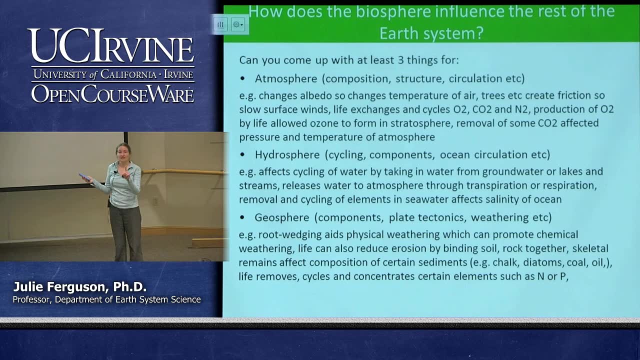 all these things I mean you can talk about with that, with your TAs, but look, I have some suggestions for you there as well. just to get you started, this will be in the lecture notes online, guys, and very quick to my last minute, so don't go anywhere. I wanted to very quickly introduce you to this. 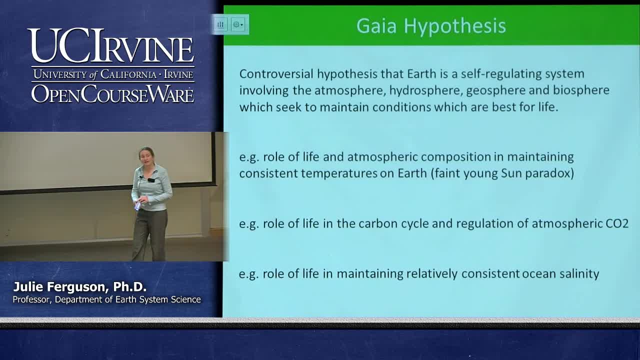 really interesting idea. it's called the Gaia hypothesis and it's really controversial and it's basically the idea that the earth could be treated as a self-regulating organism, almost, that the presence of life now is interfering with the way that the atmosphere, the hydrosphere and the